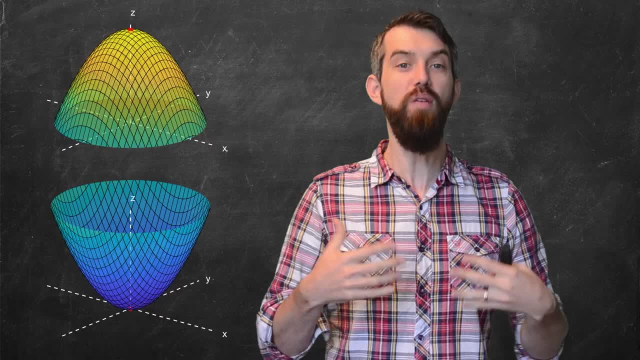 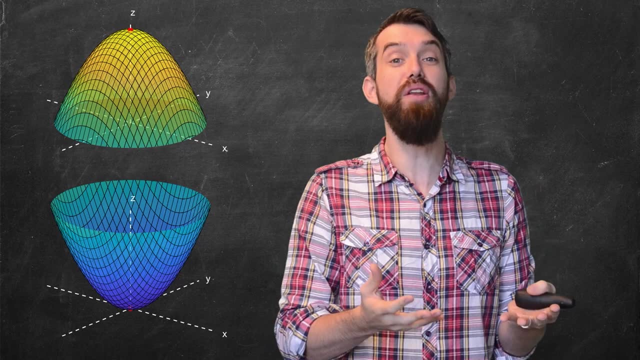 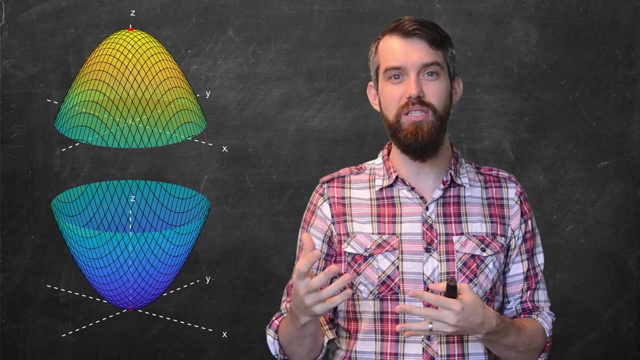 One of the most powerful applications of calculus is optimization. Indeed, if I'm given some function, how do I know when that function is going to have a maximum and how do I know when it's going to have a minimum? However, what we're going to do in this video is look. 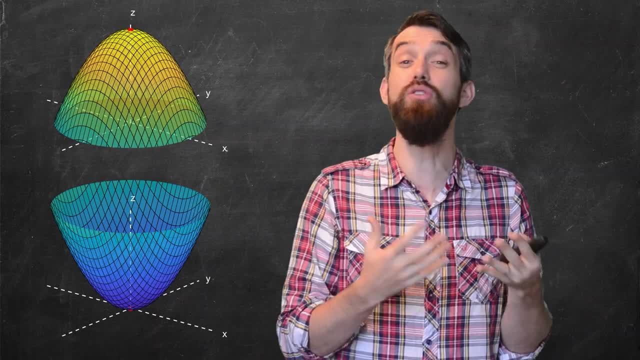 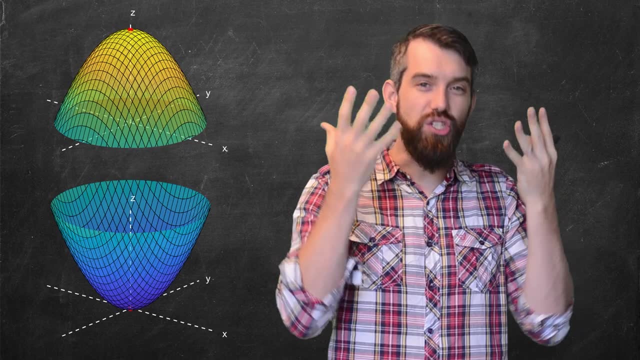 at a special type of optimization, a special type of trying to find maximums and minimums. It's when I ask you to find the maximum or the minimum, but I give you a constraint, I give you a restriction. For instance, consider this graph: What I have is just the graph. 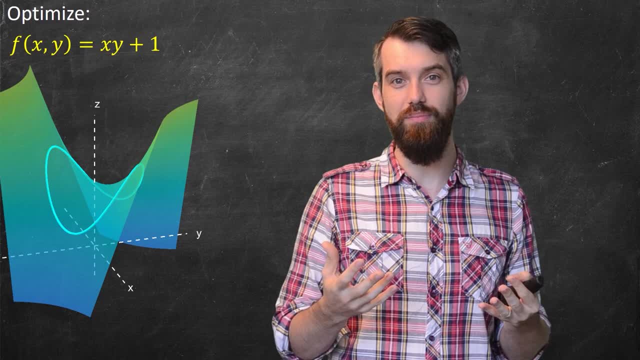 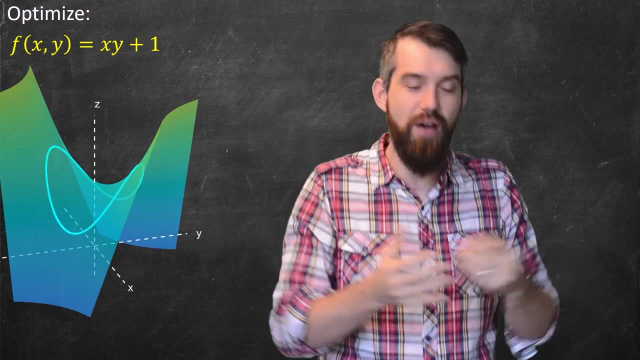 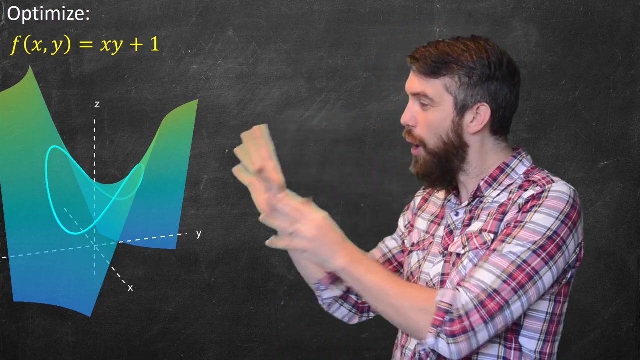 of some function, the function xy plus 1.. And the graph itself. well, it has a saddle point at the point 0, 0, but it then goes up in one direction forever and goes down in some other direction. However, if I impose a constraint, if I say it has to be on this: 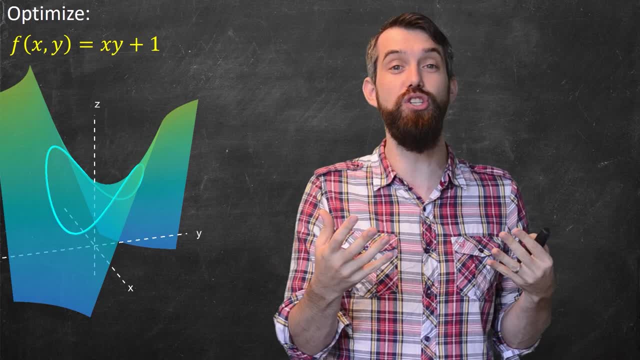 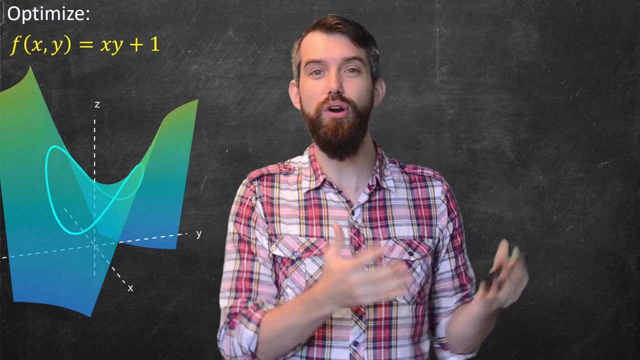 particular curve and I'm asking: what is the maximum of this function restricted to that curve? What is the minimum of this function restricted to that curve, The blue curve that I've put up here? if I look at it in the domain of my function, it's just the equation of a circle. 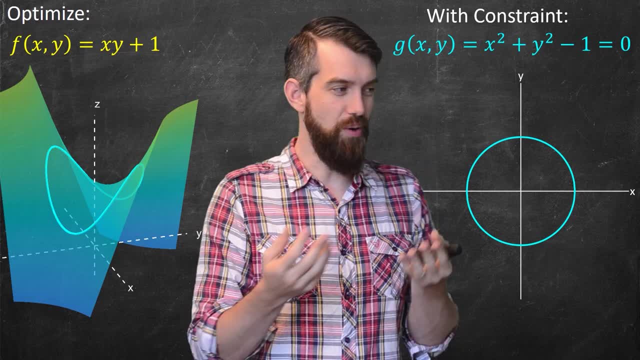 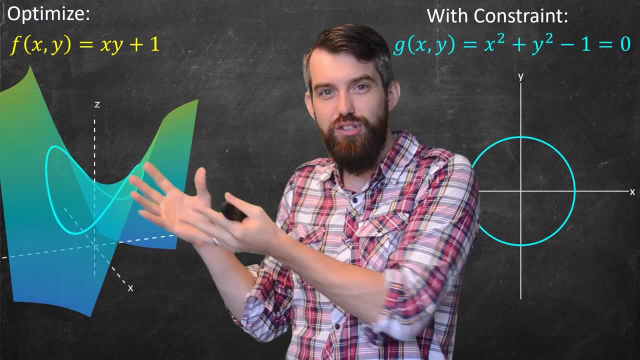 x squared plus y squared is equal to 1.. So in the domain I have a circle and I'm saying you were restricted to that circle, And then in the graph of the function you look at, well, what does the function do above that circle? And the question is: what's the maximum? 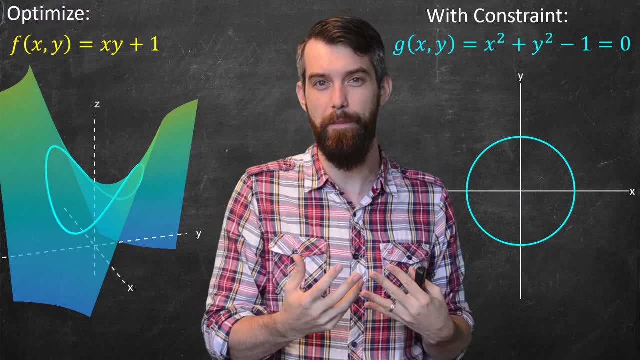 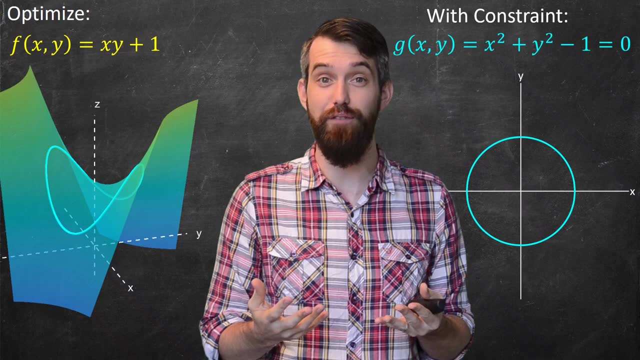 of the function of the circle and what's the minimum of this function. This video is going to talk about something called Lagrange multipliers, And Lagrange multipliers are going to give us a method to figure out the maximums of functions like these when 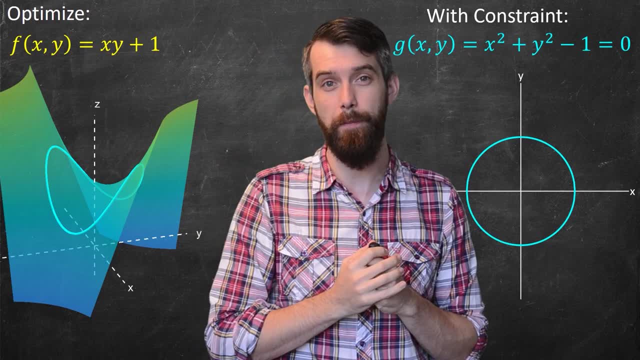 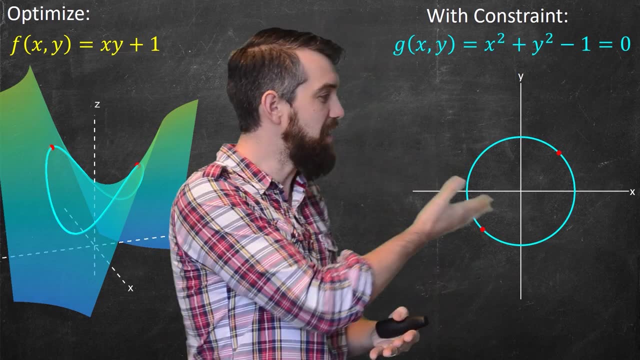 you're constrained to specific constraints, like this circle For instance. I've highlighted here in the red dots the maximums of the value of the function, constrained to live on the curve. And then in the domain, the two red dots say: well, where in the domain am I going? 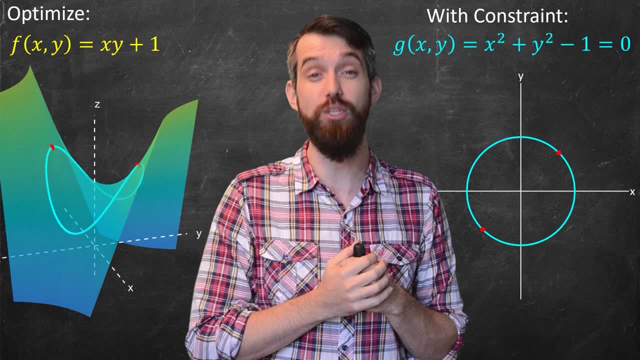 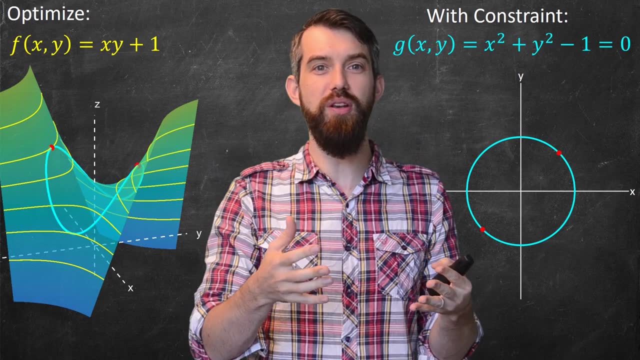 to have these maximums. Also, it looks like I have two minimums as well. To help me understand what's going on here, I put up contours on the graph of my function. Remember that what the contour is is you telling me? the height is constant, So I'm setting. 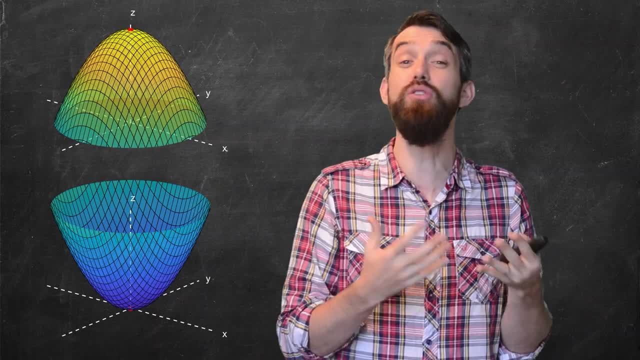 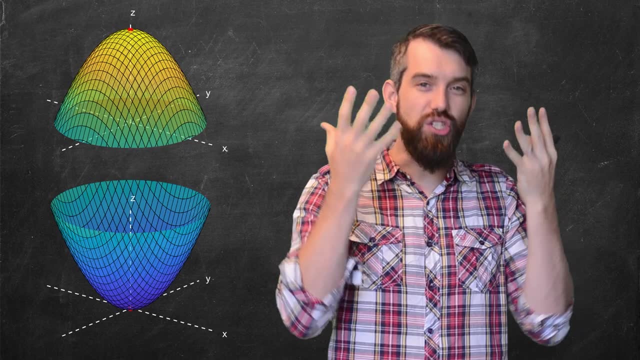 at a special type of optimization, a special type of trying to find maximums and minimums. It's when I ask you to find the maximum or the minimum, but I give you a constraint, I give you a restriction. For instance, consider this graph: What I have is just the graph. 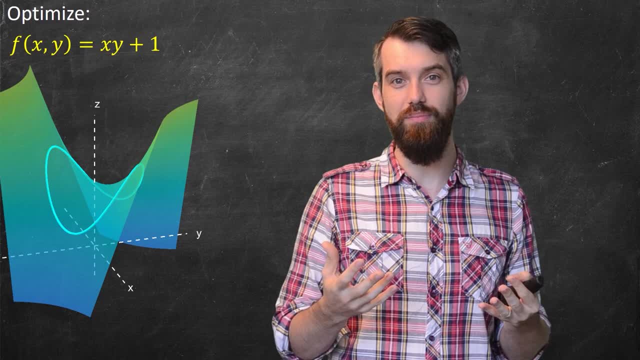 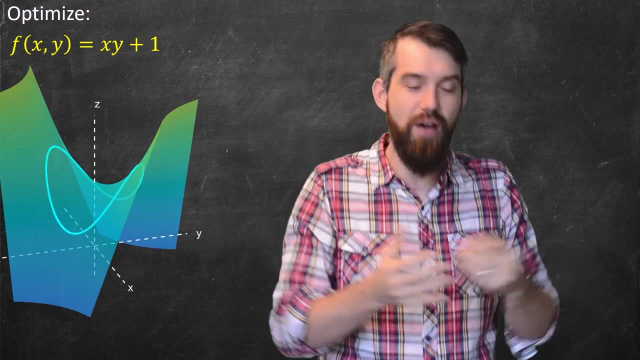 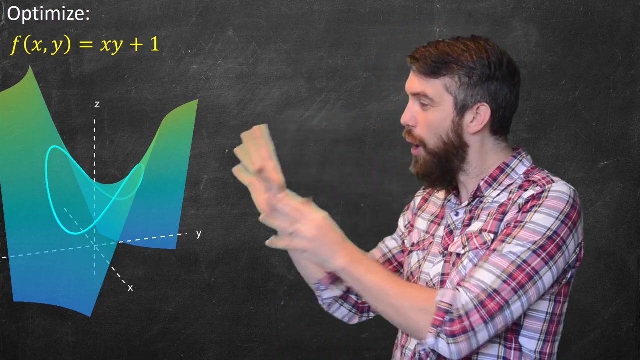 of some function, the function xy plus 1.. And the graph itself. well, it has a saddle point at the point 0, 0, but it then goes up in one direction forever and goes down in some other direction. However, if I impose a constraint, if I say it has to be on this: 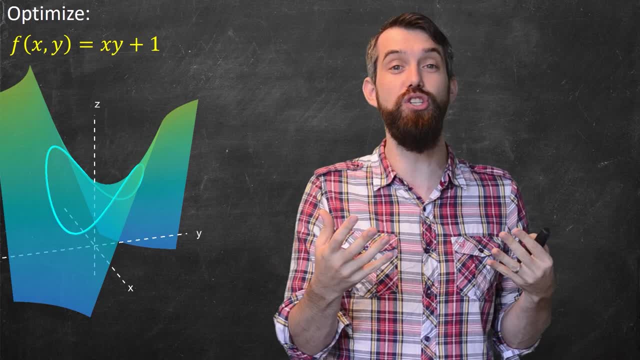 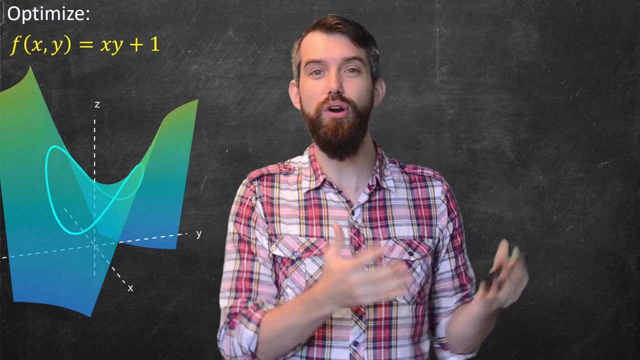 particular curve and I'm asking: what is the maximum of this function restricted to that curve? What is the minimum of this function restricted to that curve, The blue curve that I've put up here? if I look at it in the domain of my function, it's just the equation of a circle. 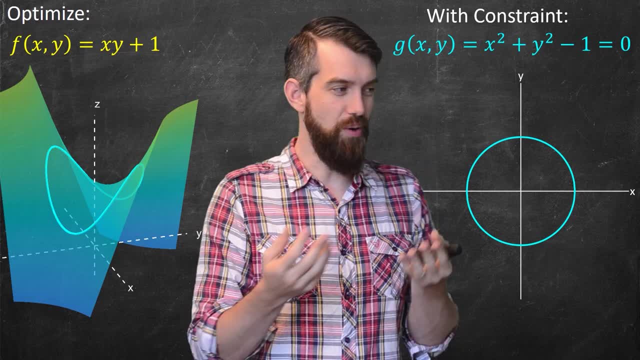 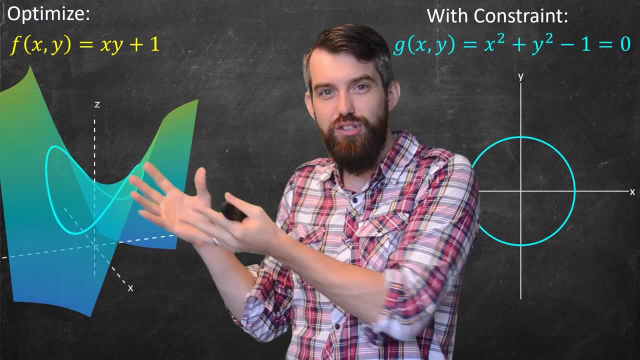 x squared plus y squared is equal to 1.. So in the domain I have a circle and I'm saying you were restricted to that circle, And then in the graph of the function you look at, well, what does the function do above that circle? And the question is: what's the maximum? 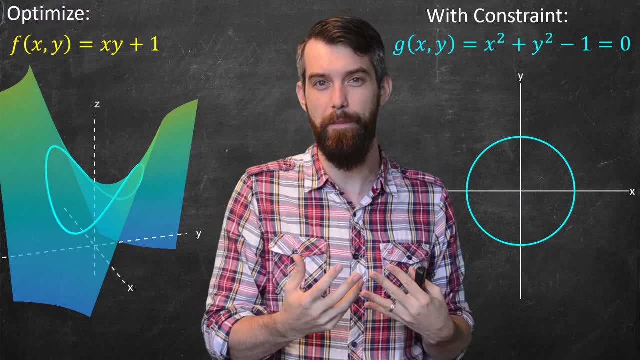 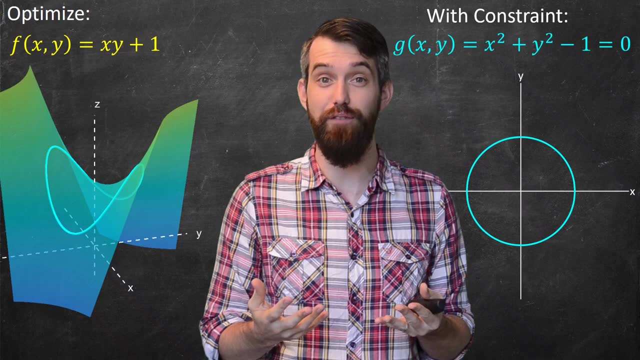 of the function of the circle and what's the minimum of this function. This video is going to talk about something called Lagrange multipliers, And Lagrange multipliers are going to give us a method to figure out the maximums of functions like these when 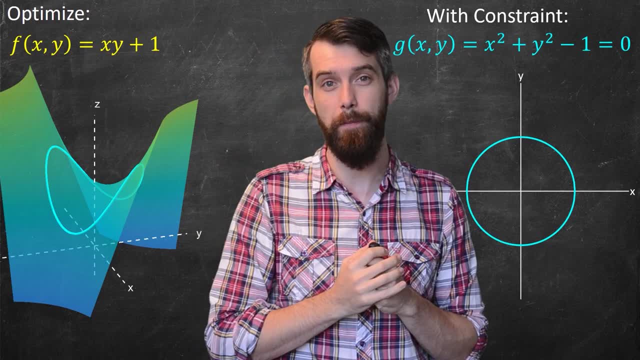 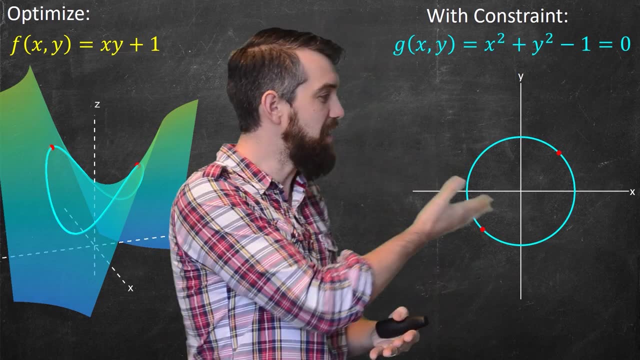 you're constrained to specific constraints, like this circle For instance. I've highlighted here in the red dots the maximums of the value of the function, constrained to live on the curve. And then in the domain, the two red dots say: well, where in the domain am I going? 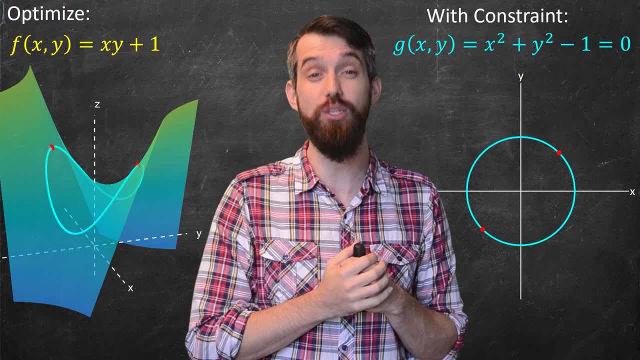 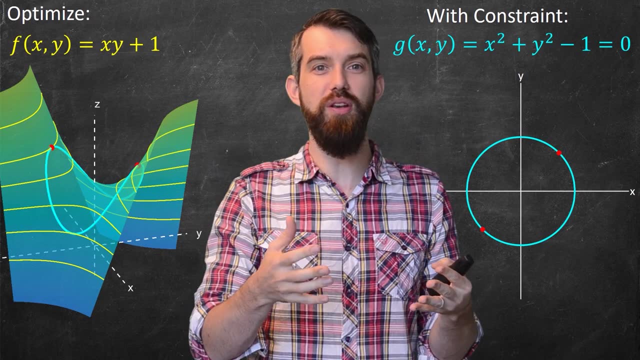 to have these maximums. Also, it looks like I have two minimums as well. To help me understand what's going on here, I put up contours on the graph of my function. Remember that what the contour is is you telling me. the height is constant, So I'm. 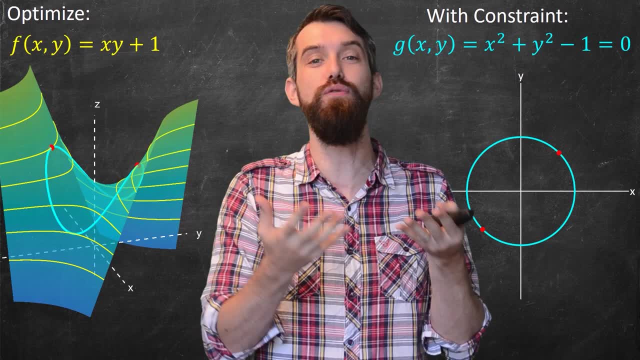 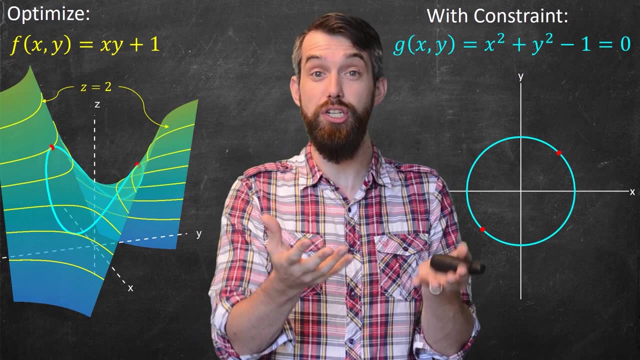 setting the function value, this x, y plus 1, equal to various constants, And then I get these resulting curves. So, for instance, if I set it equal to the value of z equal to 2, you get one curve. If I set it z equal to 1.5, you get a different curve. and so 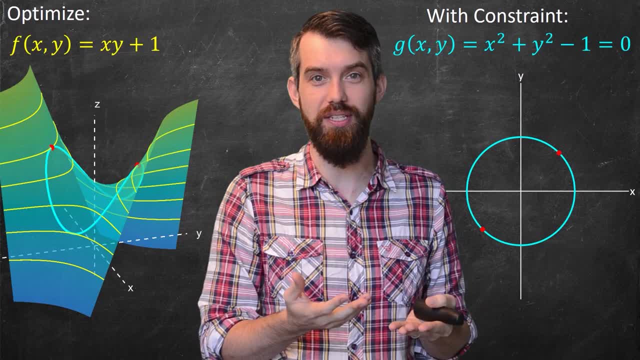 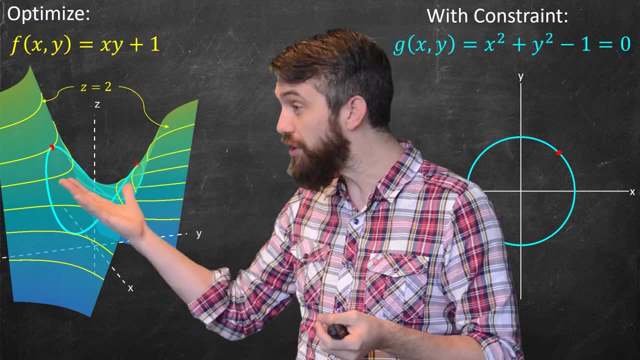 the function value this xy plus 1, equal to various constants, And then I get these resulting curves. So, for instance, if I set it equal to the value of z equal to 2, you get one curve. If I set it z equal to 1.5, you get a different curve, and so on This. 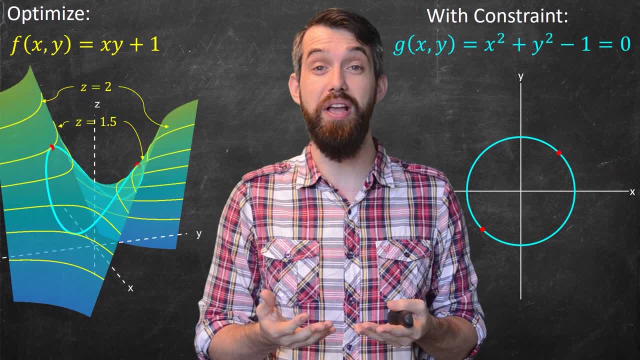 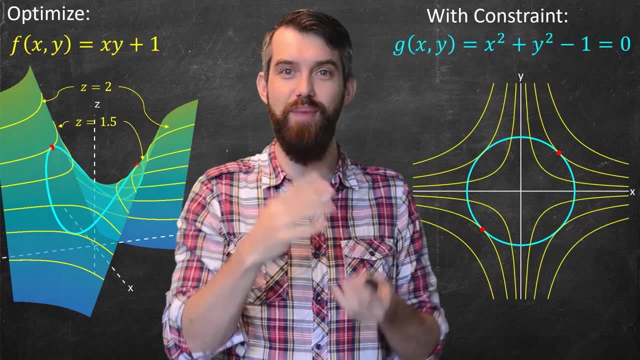 gives you a bunch of level curves, Subtitles by the Amaraorg community, And then I want you I can look at what these look like in the domain as well. Well, if I take this sort of bird's eye view and I look straight down, then I get this similar. 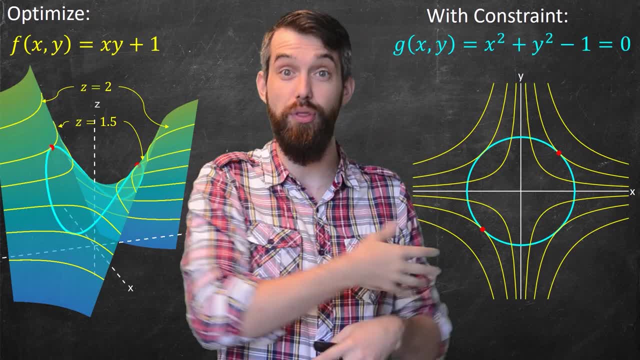 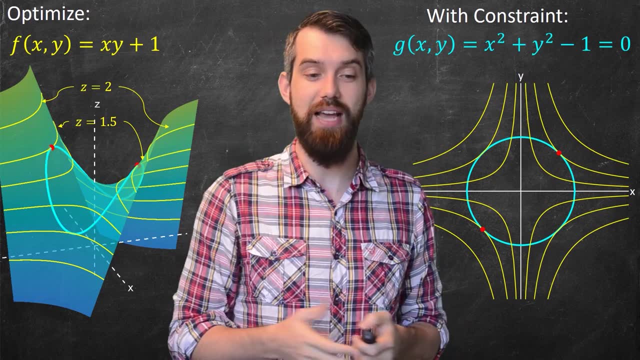 kind of effect. So I've got my blue circle, the restriction, and then the yellow curves are the level curves of the original function. For instance, if I take that z equal to 2, then I have this: z equal to 2 looks like two pieces of these curves- And z equal to 1.5. 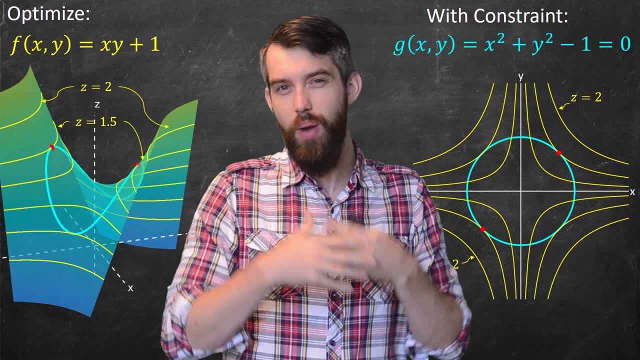 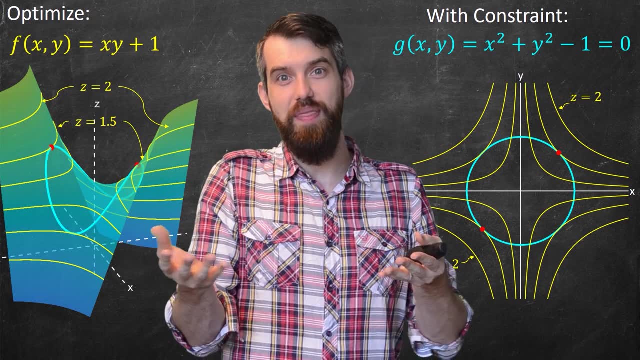 is moving in a little bit, and so forth. Subtitles by the Amaraorg community. The way I compute these is: if that the output of my function is 2, so xy plus 1 is 2,, then that means that xy is 1, which means that y is just 1 over x. So indeed, this curve. 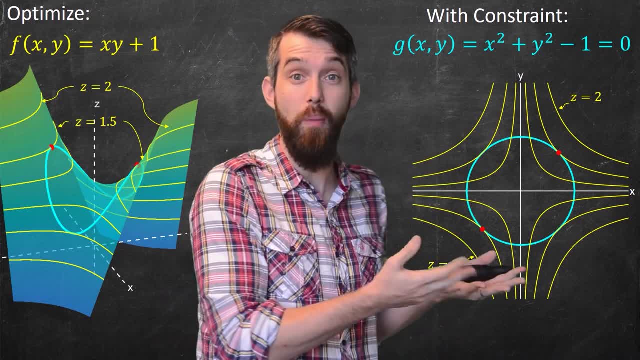 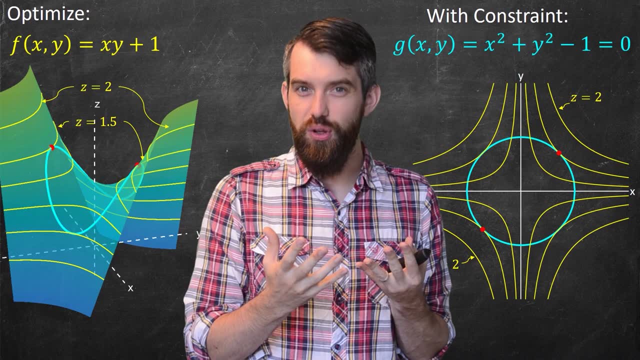 here is just representing the equation 1 over x in the domain, and that it has a height of 2.. Now, of all these different level curves, one of them is special. One of these level curves only just barely touches the restriction. Here I'll focus just a little bit on the 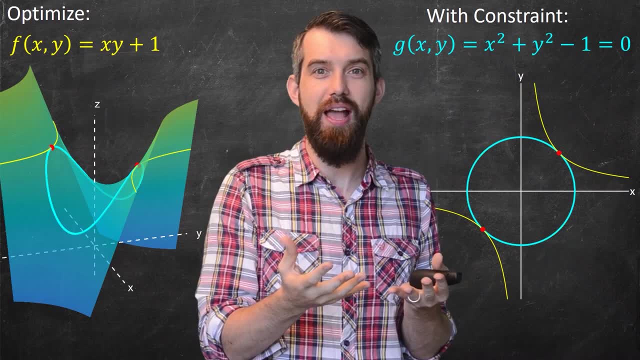 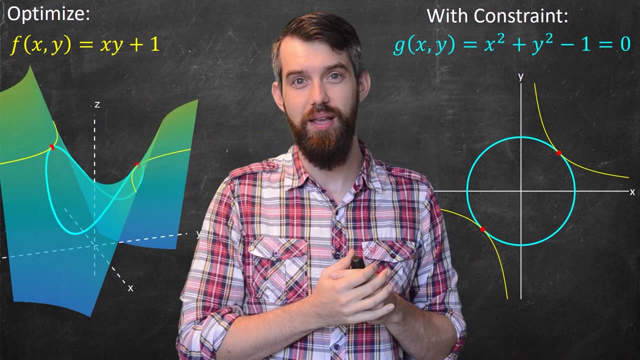 restriction. So I'll focus just in on this one. This particular level curve has the property that this level curve goes right through what looks to be the maximum of this function And indeed, if I look at what happens down in the domain that level curve, it comes. 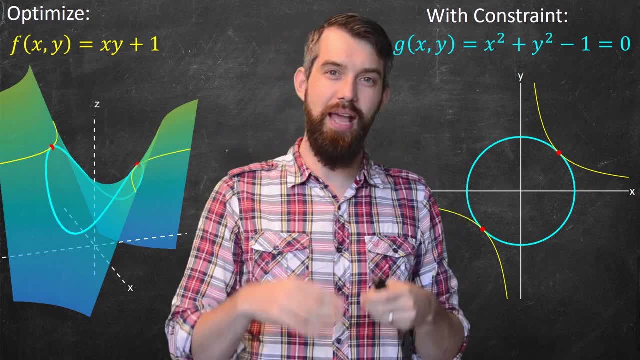 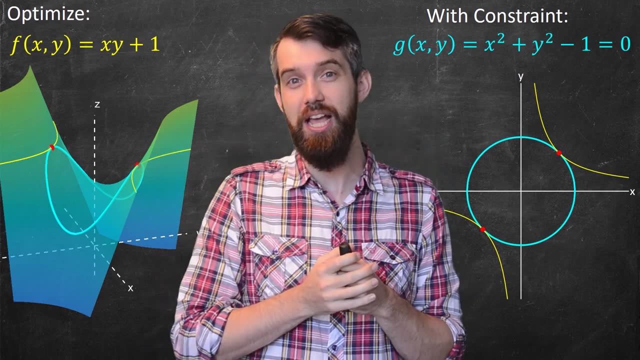 along and just barely kisses the constraints And this restriction, that I'm choosing the particular level curve that comes in and just barely touches it, that that's going to be my candidate to be a maximum or minimum. Well, if it just barely touches the restriction, 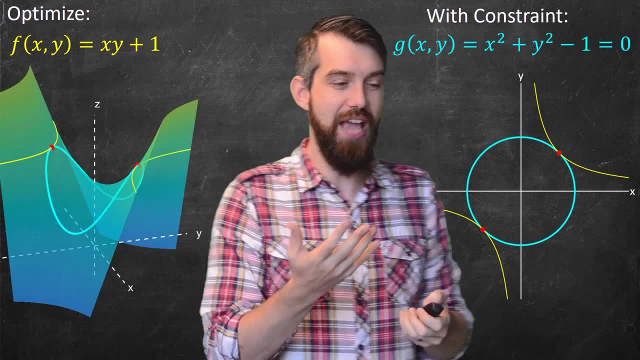 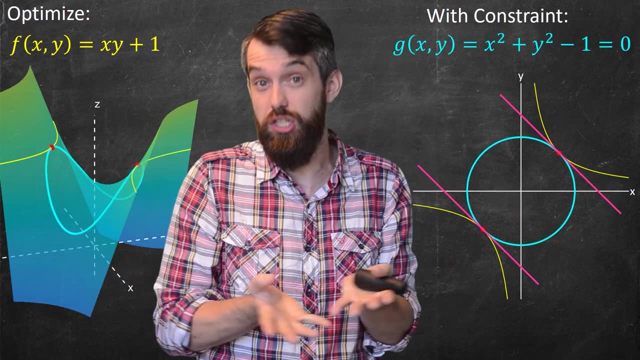 if it just barely touches it. it means something about the equation of tangent lines In particular. what it means is that the equation of the tangent line to the constraint, the equation that's just a circle, the x squared plus y squared equal to 1, that's got a tangent line. 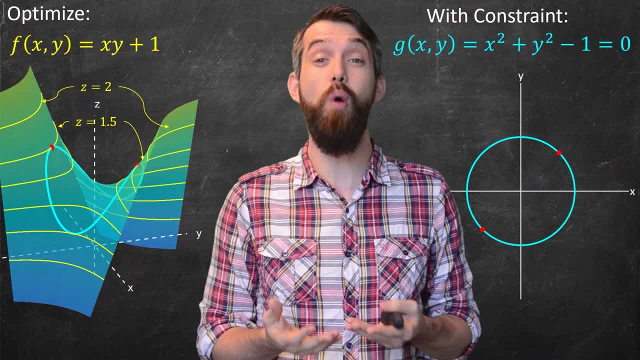 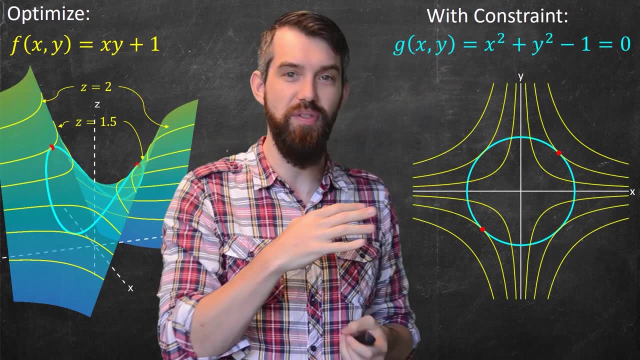 on. So I've got a bunch of level curves And then I want to. I can look at what these look like in the domain as well. Well, if I take the sort of bird's eye view and I look straight down, then I get this similar kind of effect. So I've got my blue circle, the restriction. 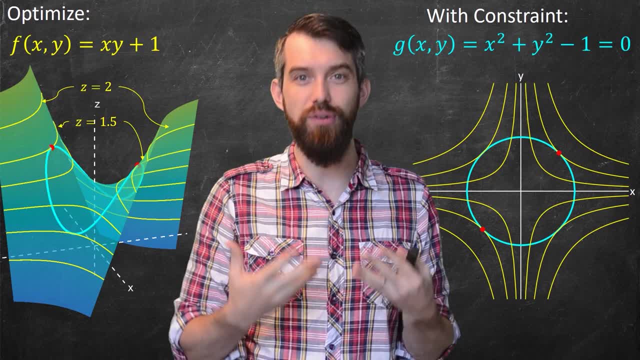 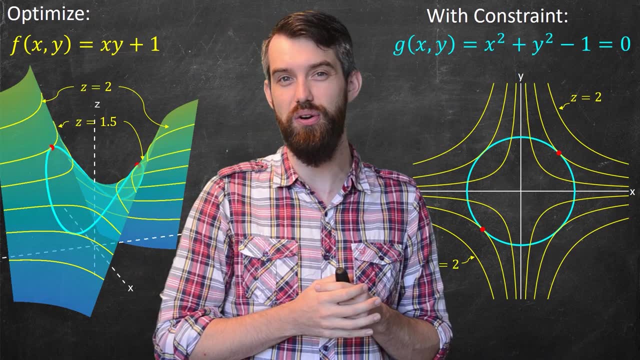 and then the yellow curves are the level curves of the original function. For instance, if I take that z equal to 2, then I have this: z equal to 2 looks like two pieces of these curves And z equal to 1.5 is moving in a little bit, and so forth. 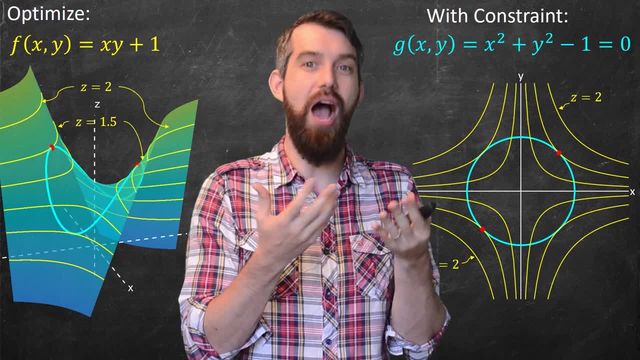 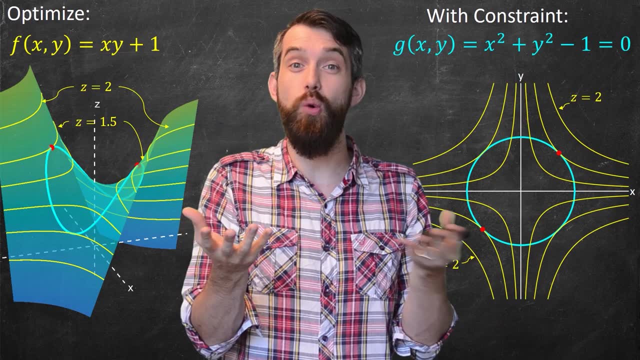 Indeed, the way I compute these is: if that the output of my function is 2, so x, y plus 1 is 2,, then that means that x- y is 1, which means that y is just 1 over x. So indeed, 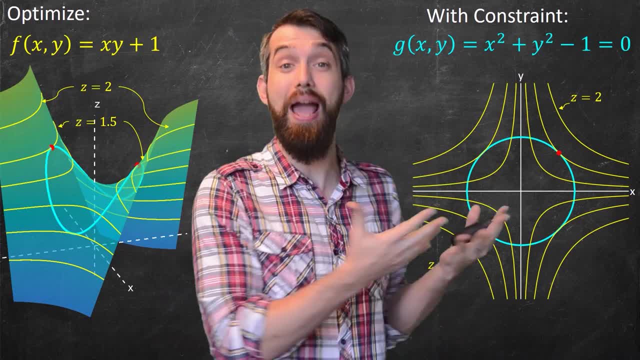 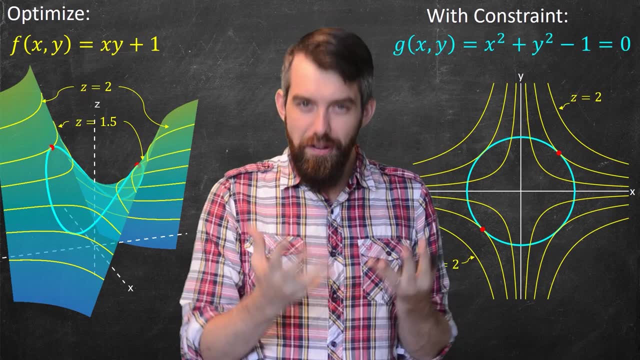 this curve here is just representing the equation 1 over x in the domain, and then it has the height of 2.. Now, of all these different level curves, one of them is special. One of these level curves only just barely touches the restriction Here, only just barely touches. 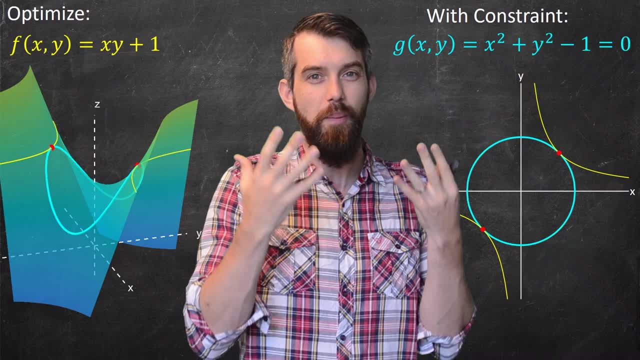 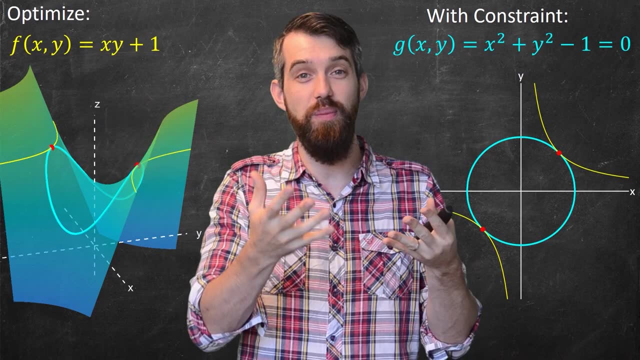 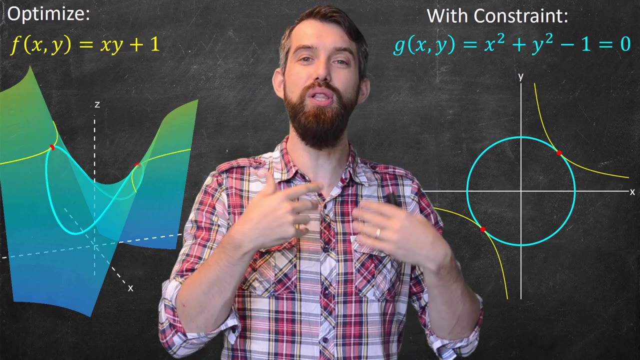 the restriction. I'll focus just in on this one. This particular level curve has the property that this level curve goes right through what looks to be the maximum of this function And indeed, if I look at what happens down in the domain that level curve, it comes along and just 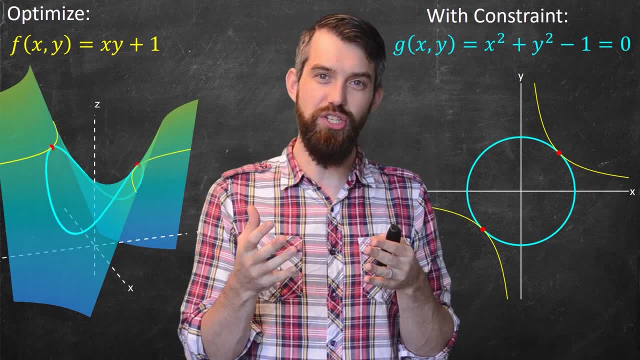 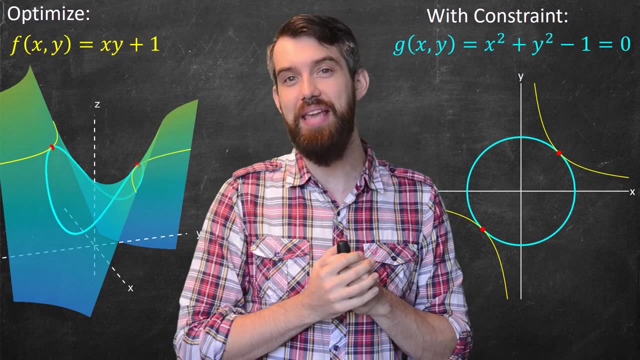 barely kisses the constraints And this restriction that I'm choosing, the particular level curve that comes in and just barely touches it, that that's going to be my candidate to be a maximum or minimum. Well, it's going to be a minimum. It's just barely with the same extent that the whole line of height, even if they're 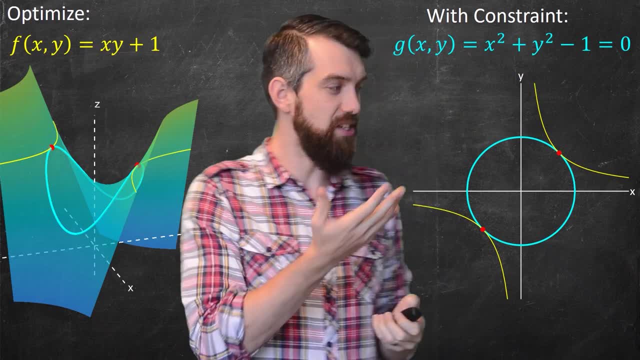 seen from Right here. I'm just going to come in on this and you can see that in my notation, say, after I write down the lot, the total length of the rotation is me for that line, but that all of the copying- I'll take into account that I'm justいい- is only for money to pay off. 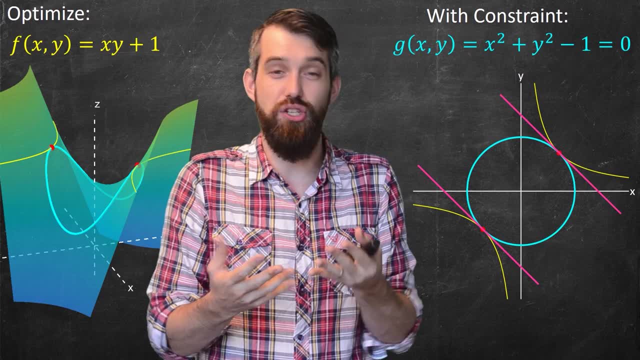 in terms of the integration of oututer space, Right, But so if it just barely touches it, it means something about the equation of tangent lines in particular. what it means is that the equation of the tangent line to the constraint, the equation that's just a circle, the x modules was rise to equal to one that's going to. 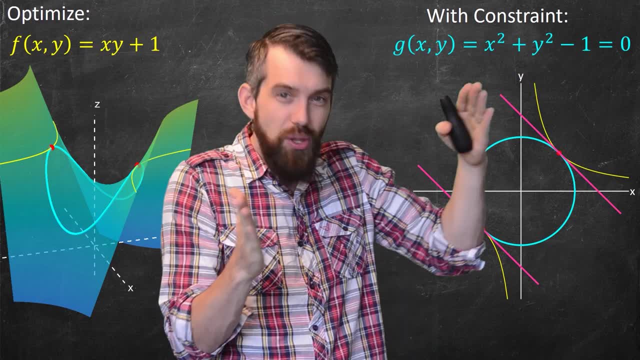 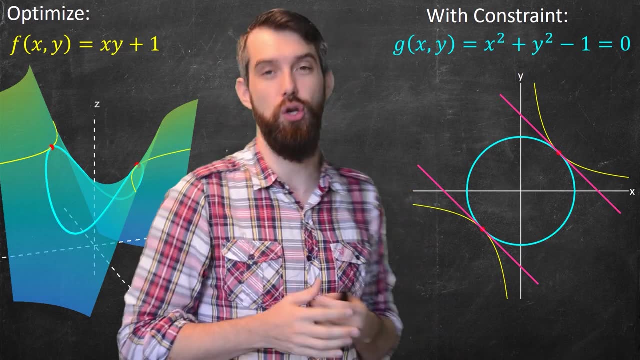 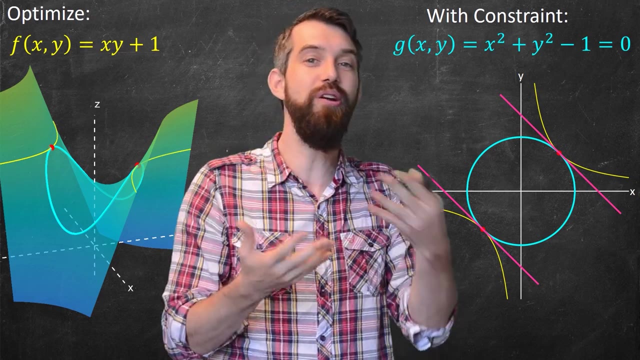 touch up line and the level curve also has a tangent line And if they come along and just meet, those tangent lines are the same thing. So at the two spots where this particular curve comes and just barely touches the constraint curve, then the tangent line is shared by both of 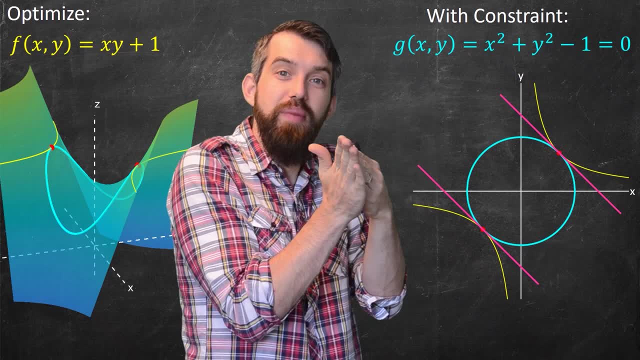 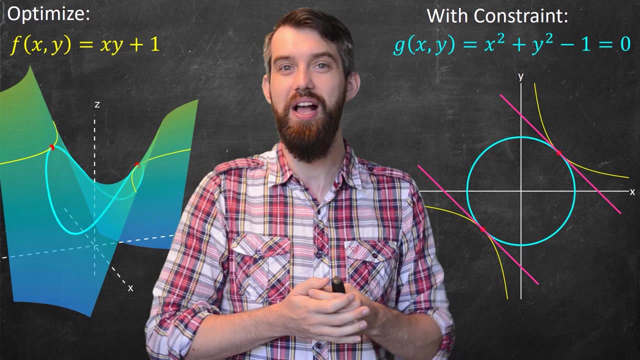 And the level curve also has a tangent line And if they come along and just meet, those tangent lines are the same thing. So at the two spots where this particular curve comes and just barely touches the constraint curve, then it's just barely touching the constraint. 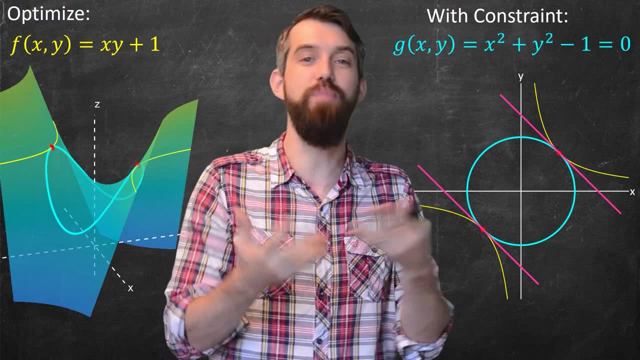 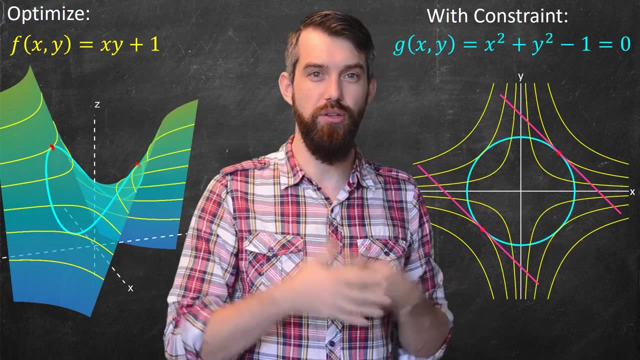 curve And the tangent line is shared by both of these curves. Indeed, if I put all the curves back on here again, you see that this case is pretty special. You'll see that some of the level curves don't intersect at all In most cases. they're just not relevant. They 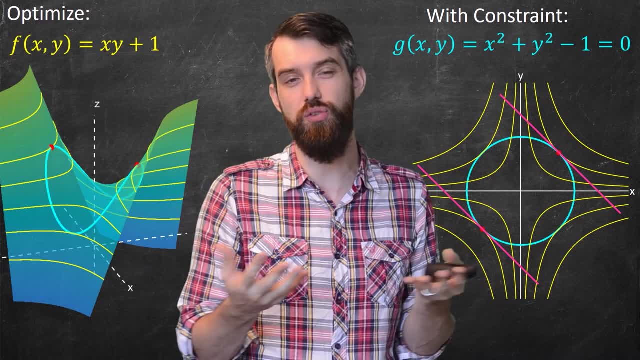 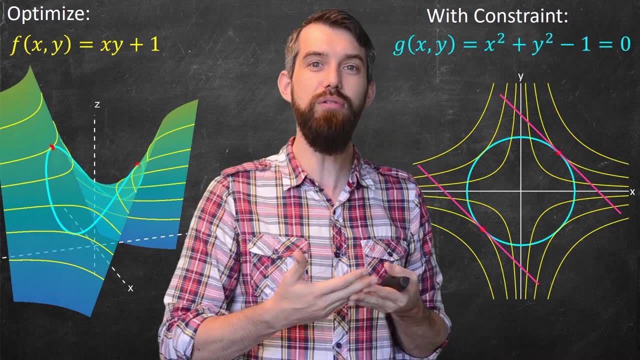 can't be part of that constraint, They're not even on the constraint. And then some of the level curves. they come in and they intersect at multiple places, But those values have lower values than the one that just comes and touches it at the one spot, If you imagine. 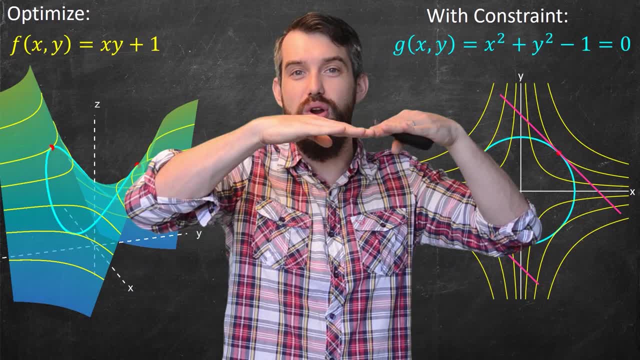 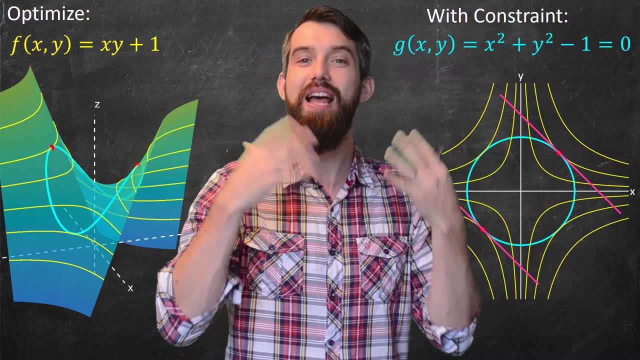 sort of continuously varying the height as you move. your level curves up. well, as you go up and up and up and up, at one point you just finally stop being subject to it. Indeed, if I took that special one, the one that's just come along, and just kissed it, if I moved it even, 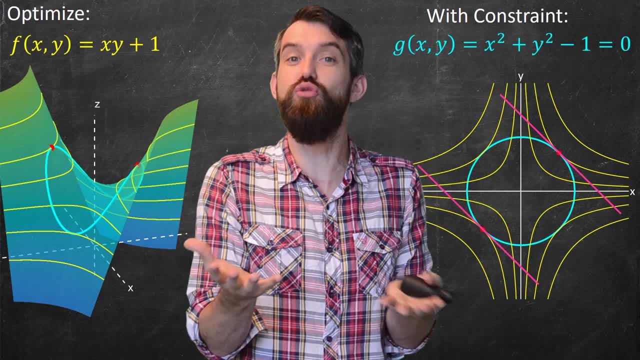 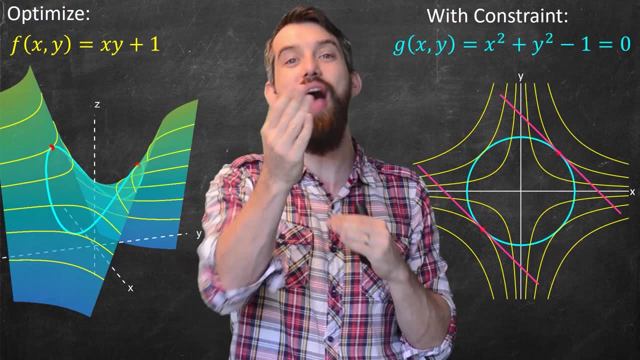 a little bit higher. it would no longer intersect the constraint in any way, It would no longer be relevant. So the one particular level curve that just comes and kisses it, that's going to be your candidates for maximums And indeed, as we can see here, we also have minimums. 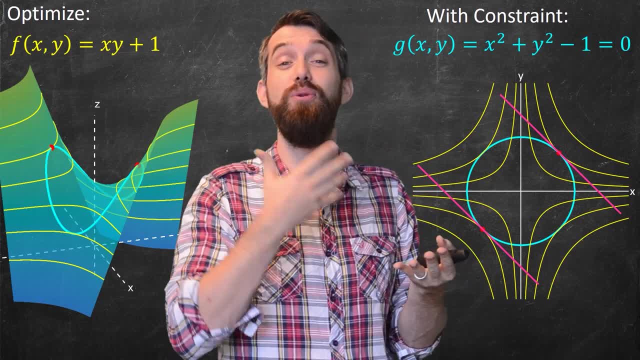 where it just comes and kisses it And the other level curves. they're just going to be your candidates for maximums And indeed, as you can see, here we also have minimums. that's going to be your candidates to be minimums. 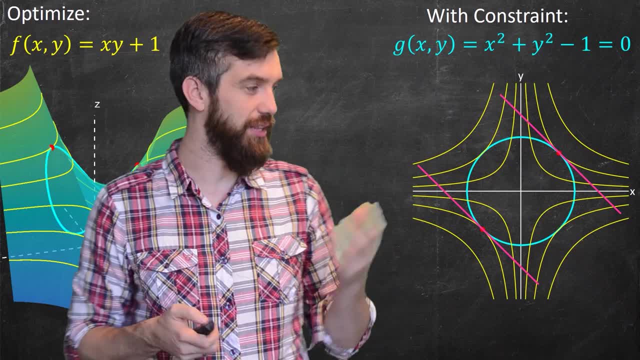 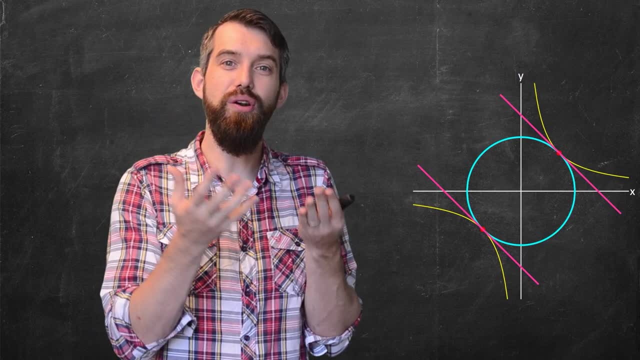 Ok, nonetheless, lets take this geometry and try to study it a bit more algebraically. so I'm going to return back to the simplified picture And what I want to notice is that they share a tangent line. then their normals are also related. For example, let me look: 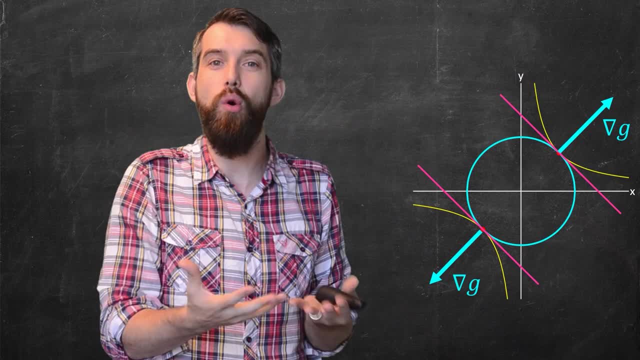 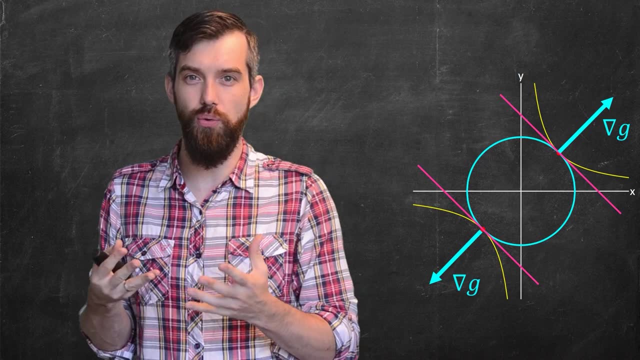 at this constraint, the blue circle. here There is a normal to that curve and you may recall the gradient vector is always is normal to 11. curve. So at these two points the gradient of g is normal to the particular level curve and indeed 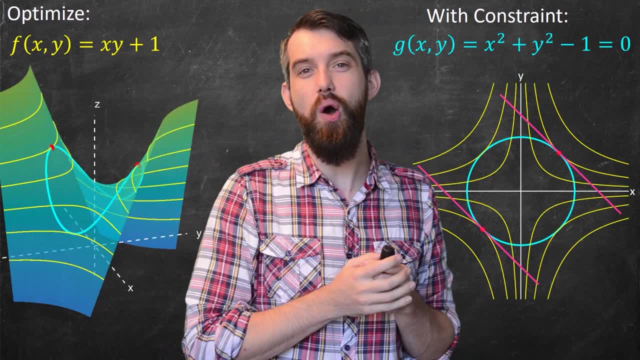 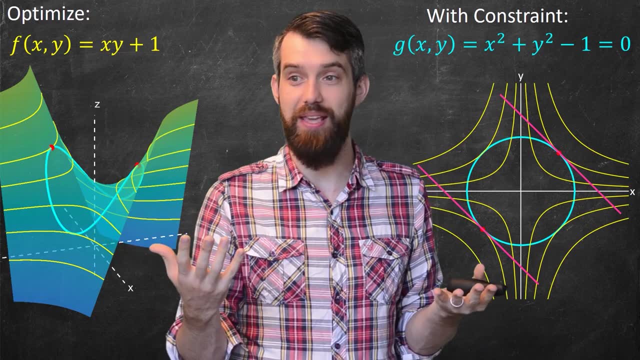 these curves. Indeed, if I put all the curves back on here again, you see that this case is pretty special. You'll see that some of the level curves don't intersect at all, in which case they're just not relevant. they can't be part of that constraint, they're not even on the constraint. And then some 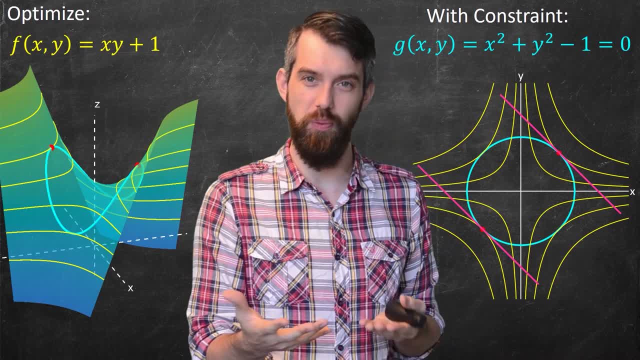 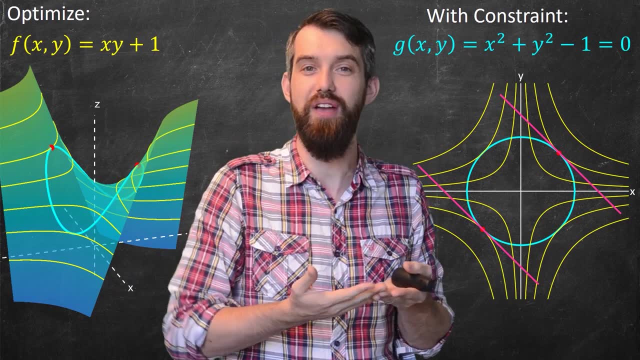 of the level curves. they come in and they intersect at multiple places, but those values have lower values than the ones that just comes and touch it at the one spot. If you imagine sort of continuously varying the height as you move your level curves up. well, as you go up and up, 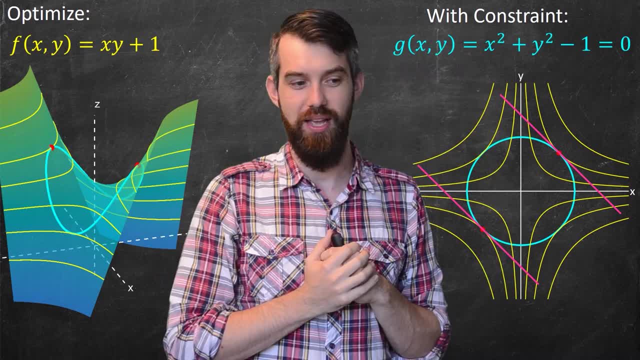 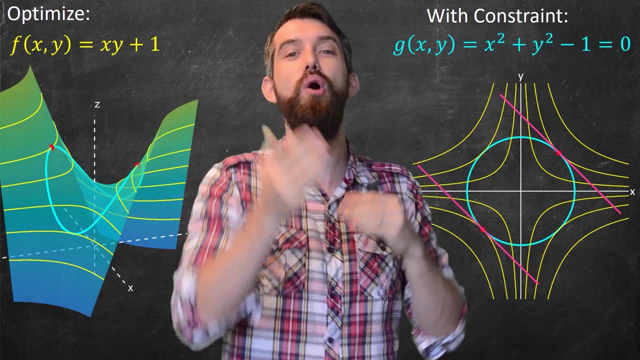 and up and up. at one point you just finally stop being subject to it. Indeed, if I took that special one, the one that's just come along, and just kissed it, if I moved it even a little bit higher, it would no longer intersect the constraint in any way, it would no longer be relevant. 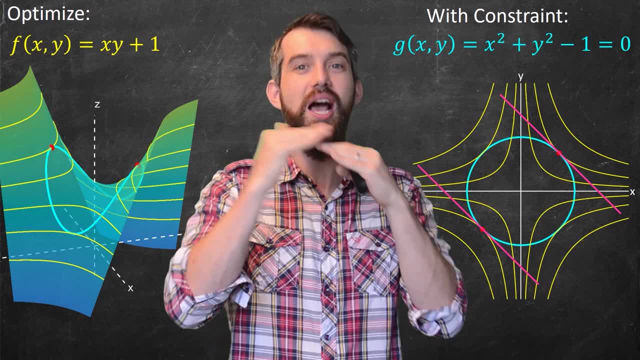 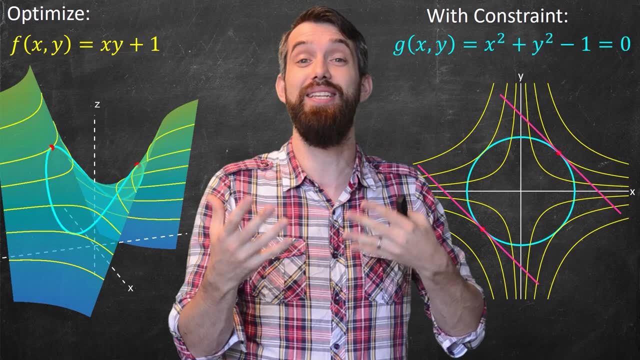 So the one particular level curve that just comes and kisses it, that's going to be your candidates for maximums, And indeed, as we can see here, we also have minimums where it just comes and kisses it in the other direction, along y equal to minus x. where it just kisses it, that's your. 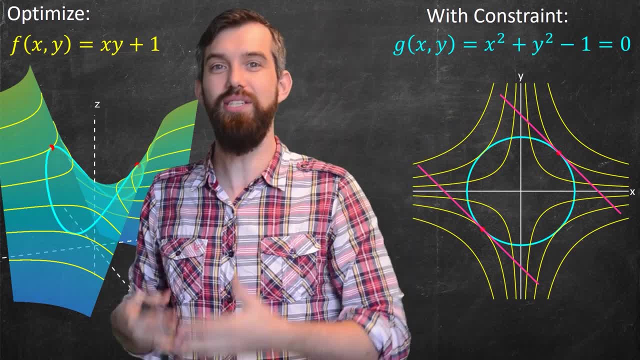 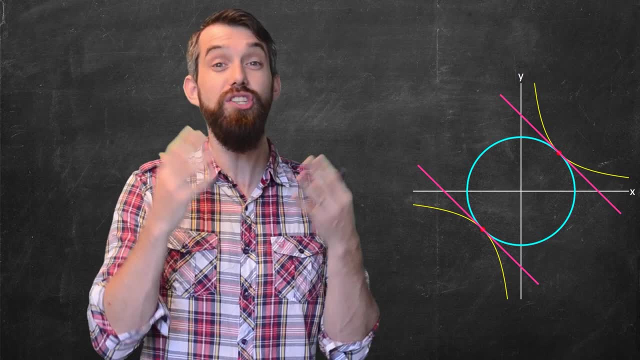 candidates to be minimums. Okay, let's take this geometry and try to study it a bit more algebraic. So I'm going to return back to the simplified picture And what I want to notice is if they share a tangent line, then their normals are also related. For example, let me look at the 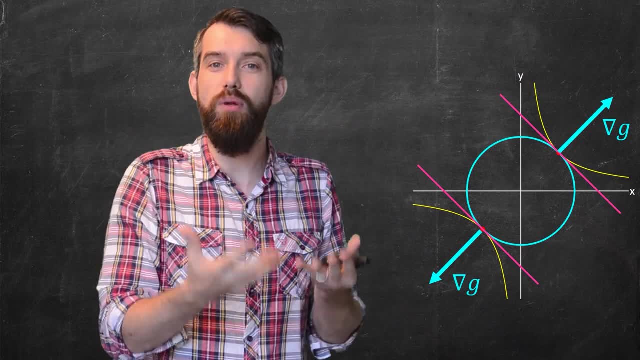 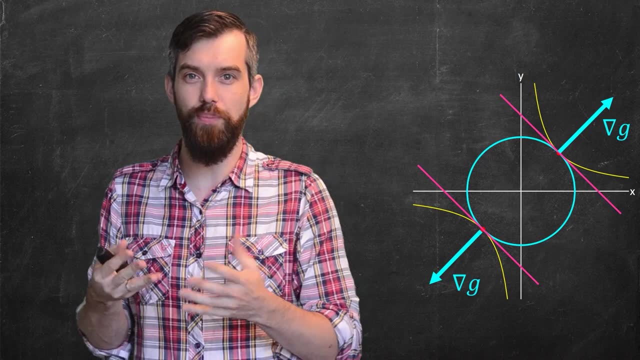 constraint, the blue circle. here There is a normal constraint- and I'm going to look at the normal- to that curve And you may recall that the gradient vector always is normal to a level curve. So at these two points the gradient of g is normal to the particular level curve And 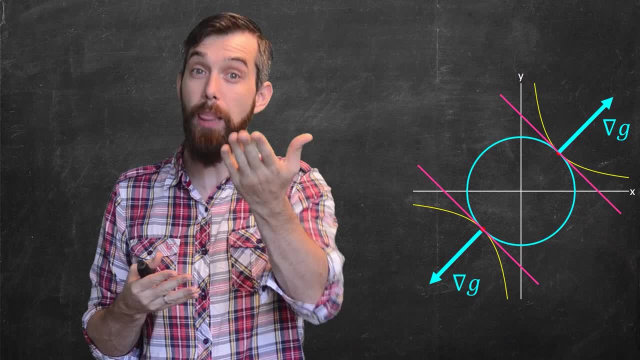 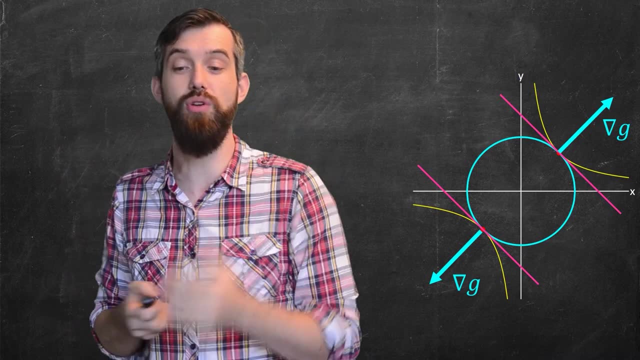 indeed it's normal to this particular tangent line. Likewise, if I look at the normals to the level curve of my function, well, I'm also going to get a gradient of f And my gradient f and gradient g, they're both normal to the same level curve. So I'm going to get a gradient of f. 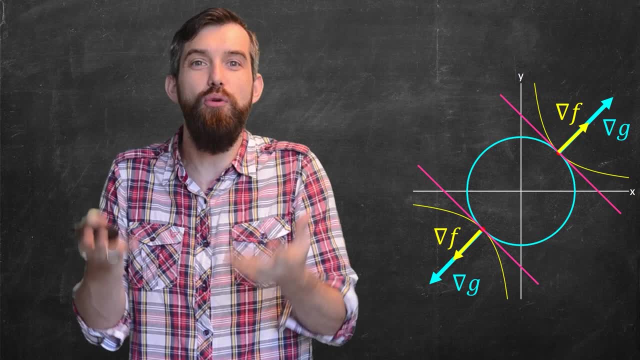 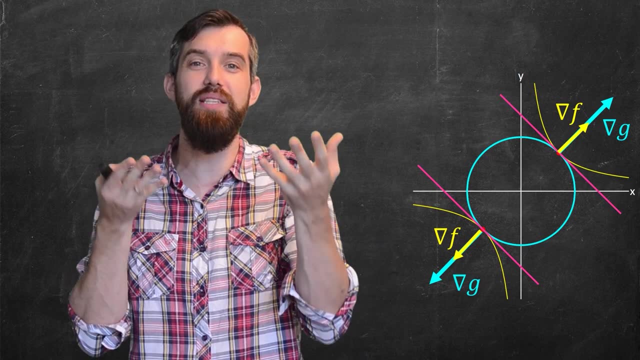 but they're both normal to the same tangent line. So the gradient of f and the gradient g are both normal to the same tangent line. And if gradient of f and gradient g are both normal to the same tangent line, what that means is they are scalar multiples of one another. The gradient of f might. 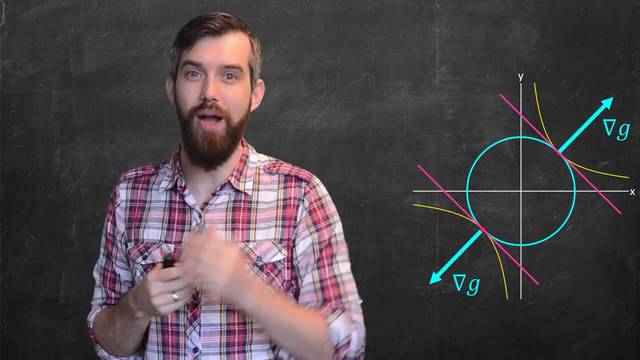 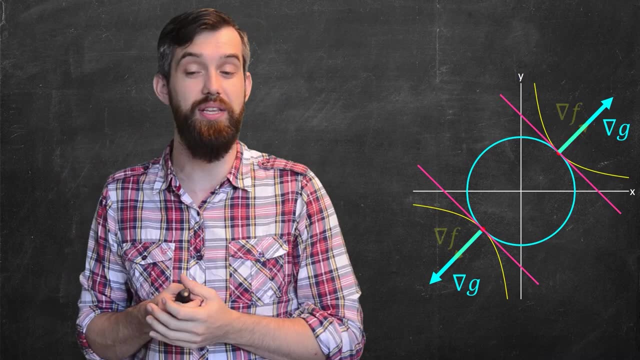 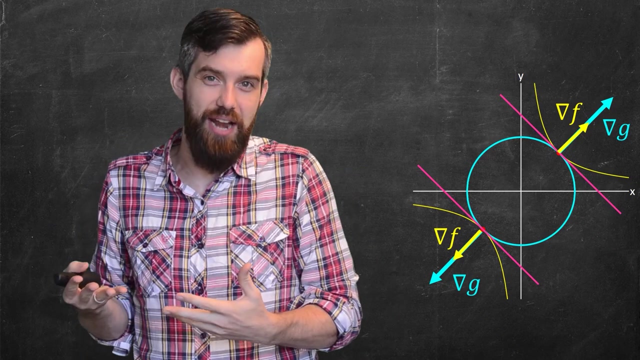 it's normal to this particular tangent line. Likewise, if I look at the normals to the level curve of my function, well, I'm also going to get a gradient of f and my gradient f and gradient g. they're both normal to the same tangent line. So the gradient of f and the gradient g are both. 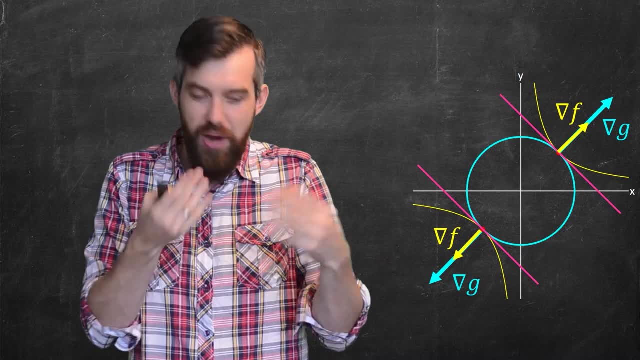 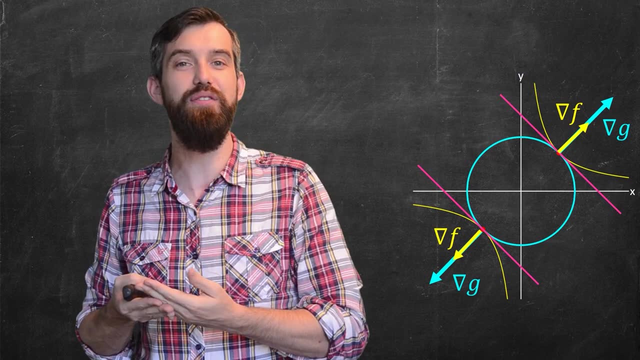 normal to the same tangent line? And if gradient of f and gradient of g are both normal to the same tangent line, what that means is they are scalar multiples of one another, That the gradient of f might be twice or one half of the gradient g, but either way it's in the same direction. 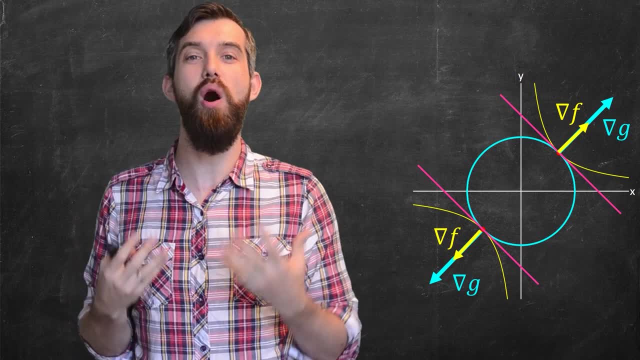 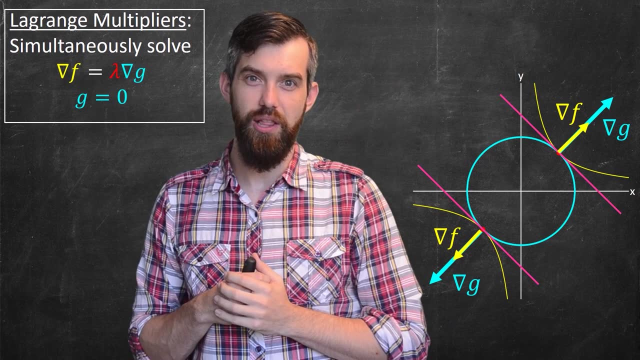 So this picture that I have motivates the Lagrange multiplier method, and it goes a little bit like this: There are two relevant equations here. The first equation is a relationship between these two gradient vectors. It's what we just talked about. geometrically, That the gradient of f 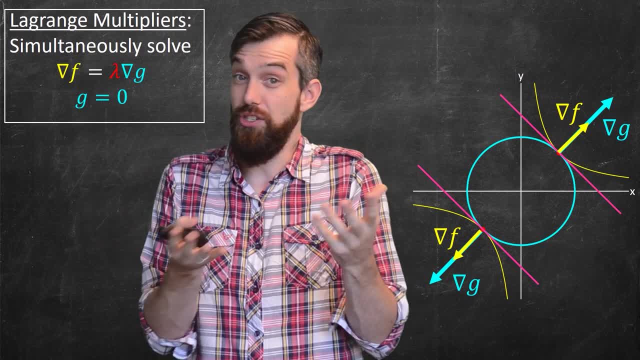 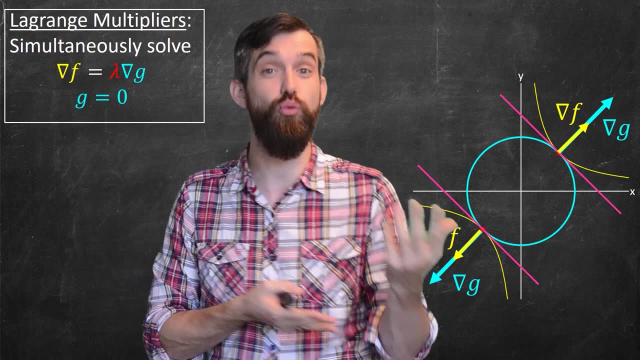 is just some multiple of the gradient of g. Lambda is just some constant and it says that these two vectors are just a multiple of the other. And then the other equation is the one we began with. We had the original constraining equation, g equal to zero. so that hasn't gone anywhere. so that's still here. 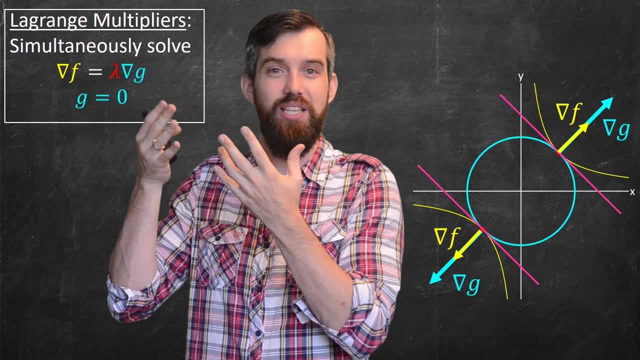 So I'm trying to maximize, and that means I got these two conditions, This business about these gradients being scalar multiples and the original constraint, the g, equal to zero. Okay, so that's the original constraint. Now let's look at the original constraint. So let's look at the. 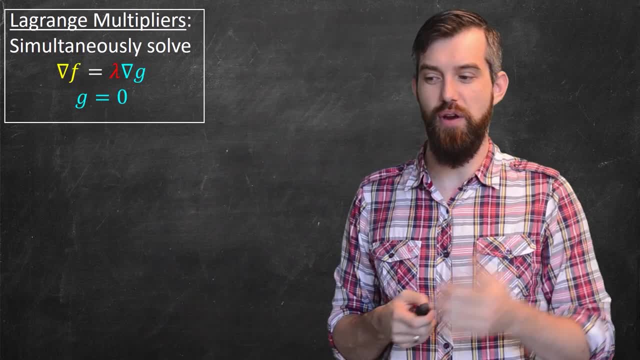 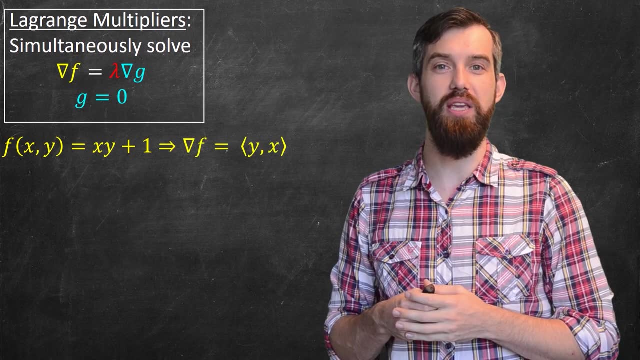 formula. Let's plug in the formulas and see what we get. So first of all we started with our function f of x equal to this xy plus 1.. That means that my gradient of that is just going to be yx. The gradient is the partial derivative with respect to x in the first component, That's just y, and 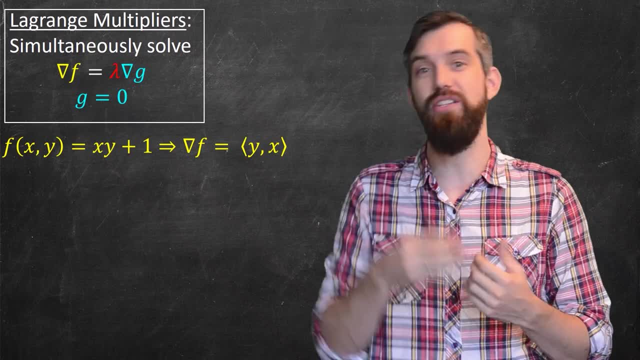 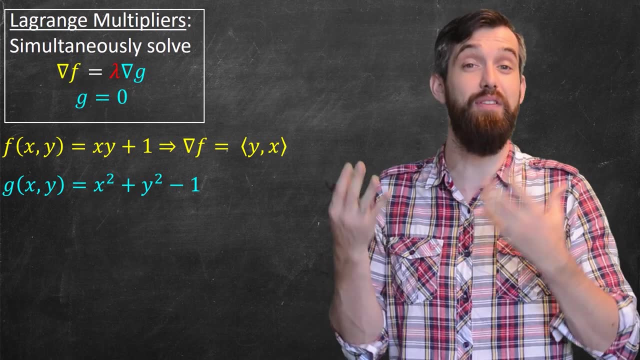 the partial derivative with respect to y in the second component, That's just x. Then if I look at my constraining equation, the g, I can do the same thing. What is the gradient of this? Well, again, I have to figure out the partial derivative with respect to x, Partial derivative with respect. 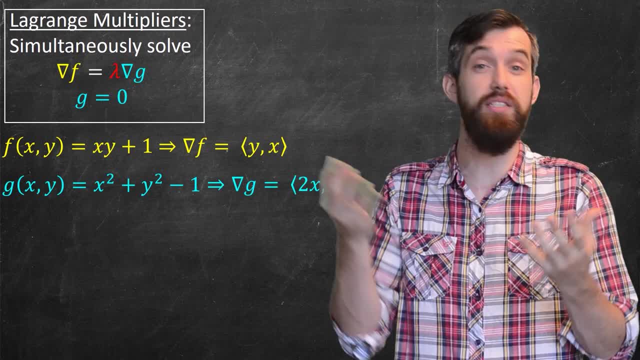 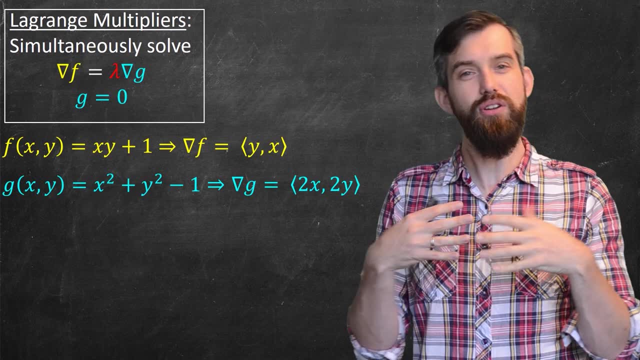 to y. What I'm going to get is 2x and 2y. Both of these gradients are easy to compute, So if I look at the two different equations that I sort of begin with, it turns out that these two equations are really. 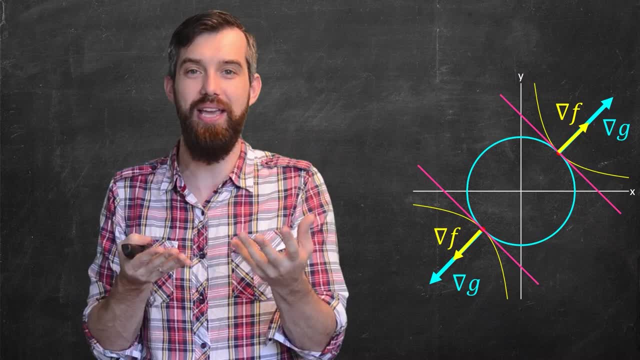 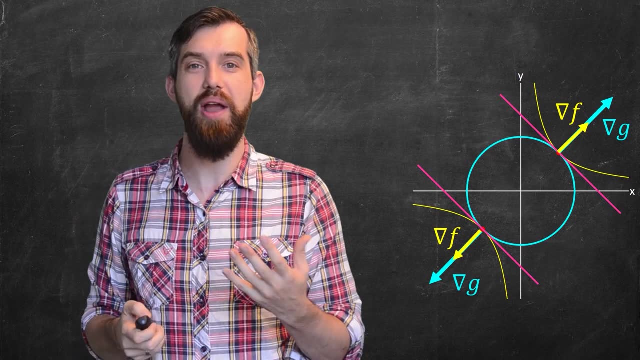 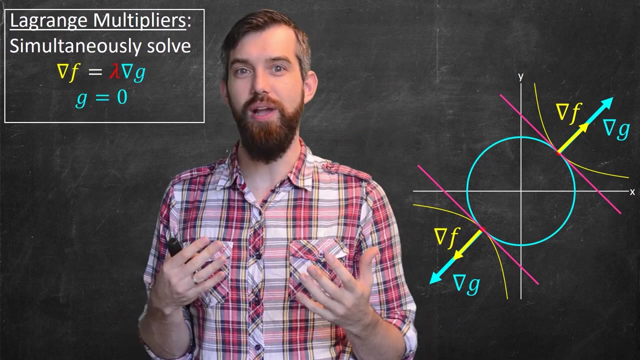 be twice or one half of the gradient g, but either way it's in the same direction. So this picture that I have motivates the Lagrange multiplier method, and it goes a little bit like this. There are two relevant equations here. The first equation is the relationship between these two gradient vectors. 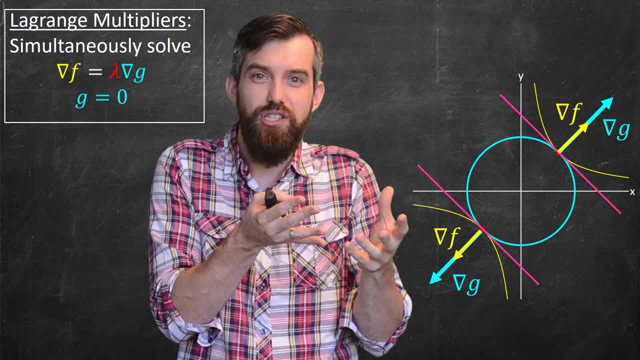 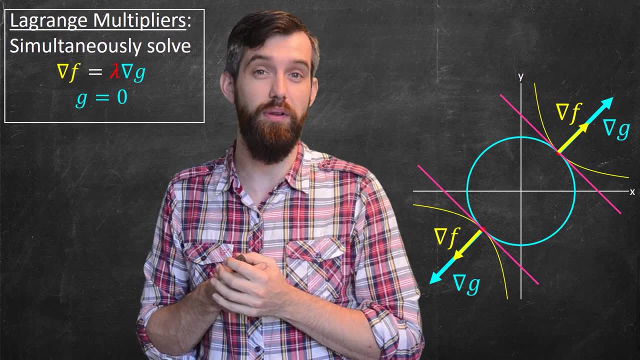 It's what we just talked about geometrically, that the gradient of f is just some multiple of the gradient of g. Lambda is just some constant, and it says that these two vectors are just a multiple of the other. And the other equation is the one we began with. We had the 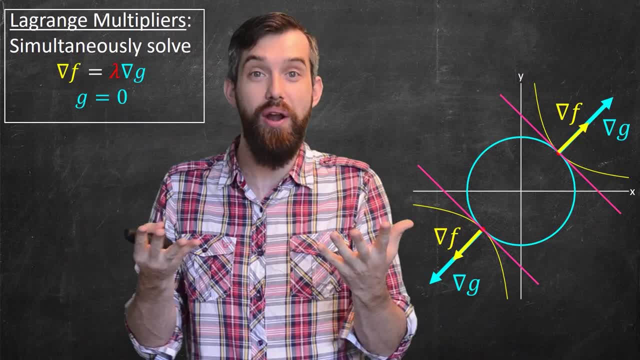 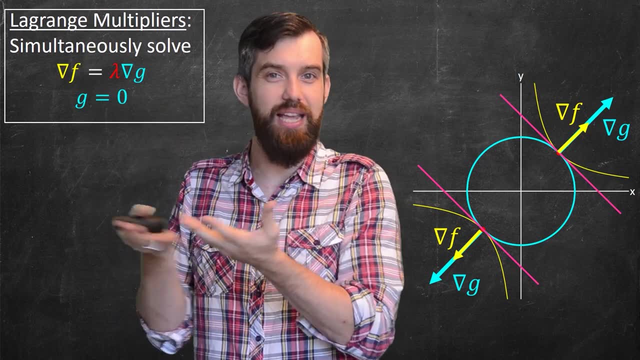 original constraining equation g equal to 0.. So that hasn't gone anywhere, so that's still here. So I'm trying to maximize and that means I've got these two conditions, this business about these gradients being scalar multiples and the original constraint, the g equal to 0. 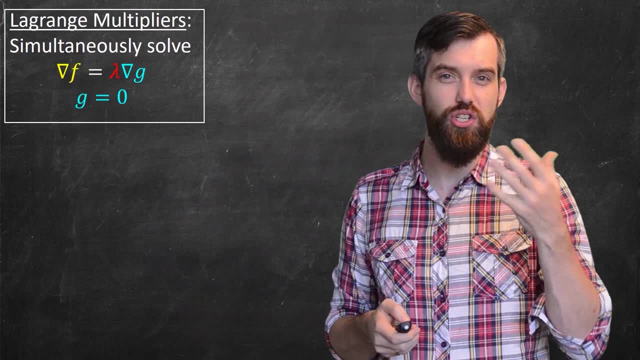 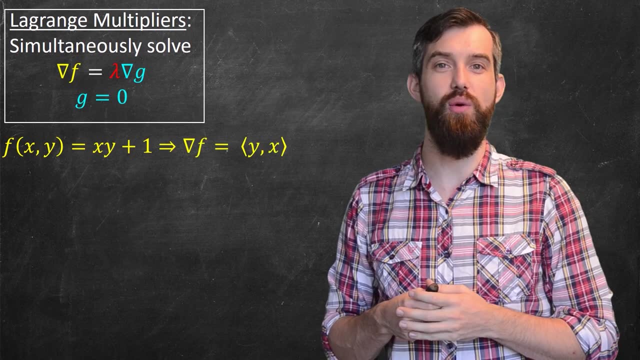 OK, so let's plug in the formulas and see what we get. So first of all, we started with our function f of x equal to this x, y plus 1.. That means that my gradient of that is just going to be y- x. 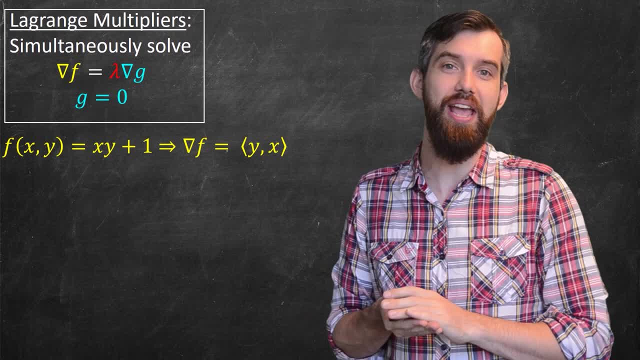 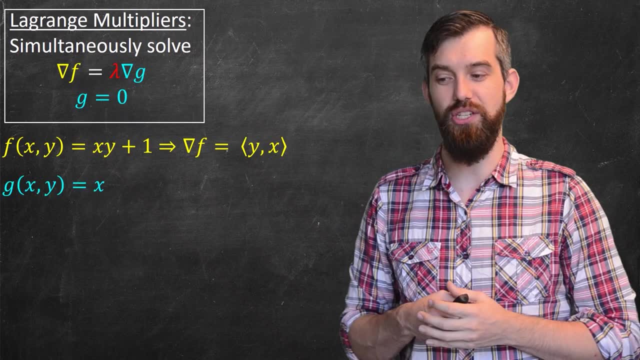 The gradient is the partial derivative of x in the first component, that's just y, and the partial derivative of x in the second component, that's just x. Then, if I look at my constraining equation, the g, I can do the same thing. What is the gradient of this? Well, again, I have to figure out the gradient of this. 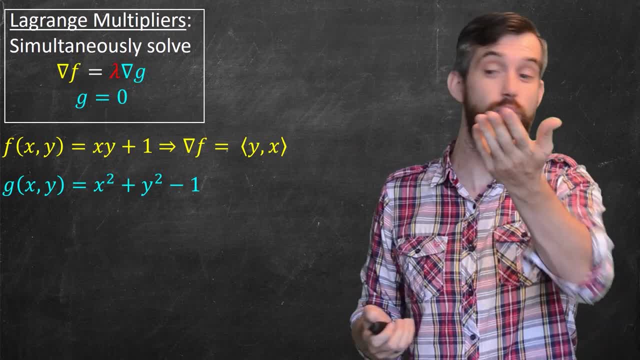 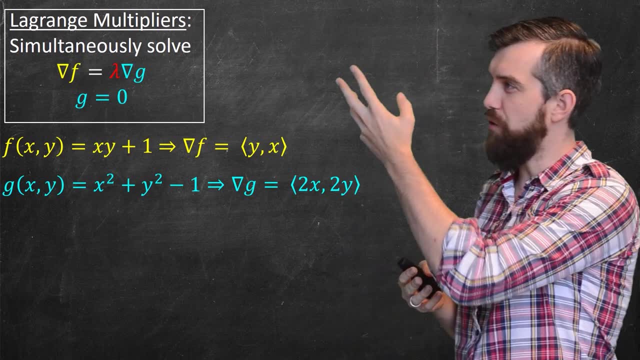 The partial derivative is respect to x, the partial derivative is respect to y, and what I'm going to get is 2x and 2y. Both of these gradients are easy to compute. So if I look at the two different equations that I sort of begin with. 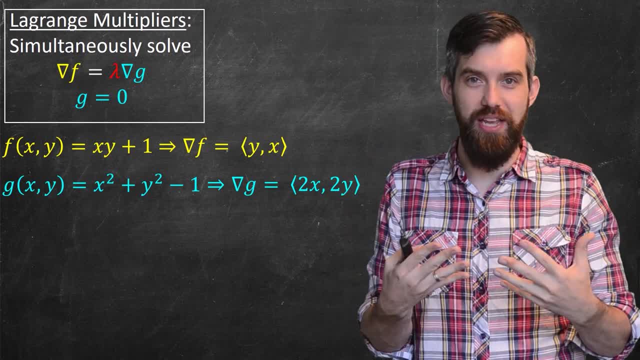 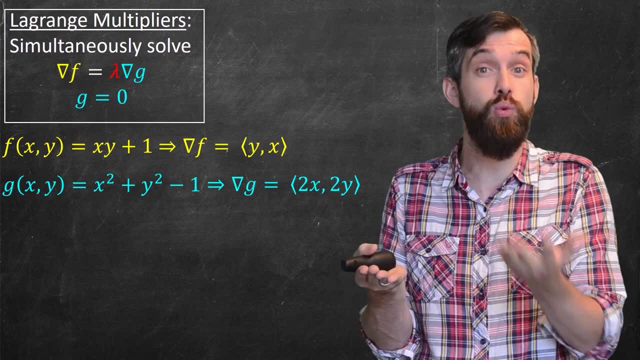 it turns out that these two equations are really three equations in three unknowns. The unknowns are the x and the y and this new thing we've come up, this lambda. So there's three unknowns: an x, y and a lambda. 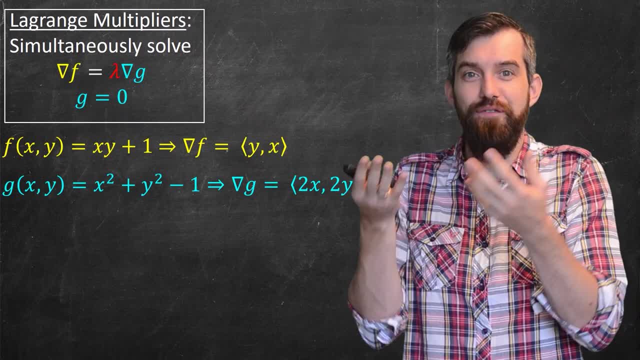 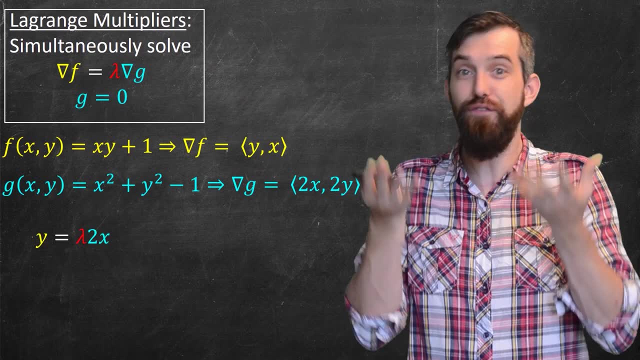 But there's really three equations, because the first equation is a vector equation. The first equation: gradient of f is lambda. gradient of g is equating two two-dimensional vectors. So the first components of that is the first component of gradient f is lambda times the first component of gradient g. 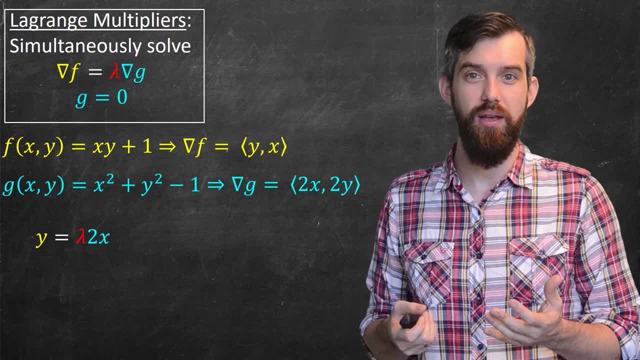 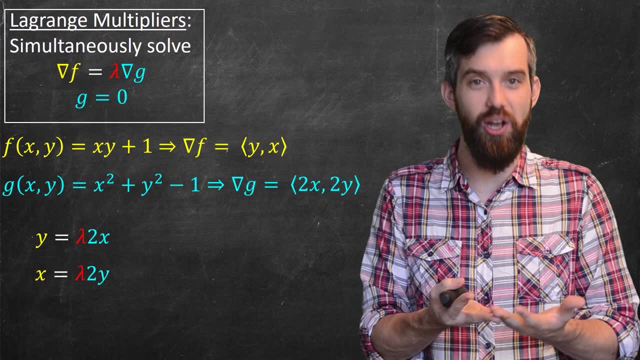 In other words, just y equals lambda times 2x. Comparing the second coordinates of this now I'm saying x is lambda times 2y. So the second component of gradient of f is equal to lambda times the second component of gradient of g. 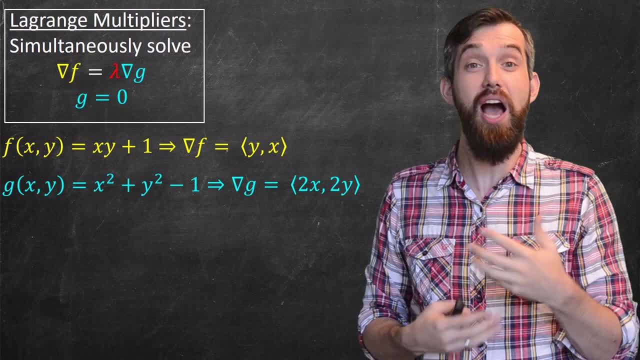 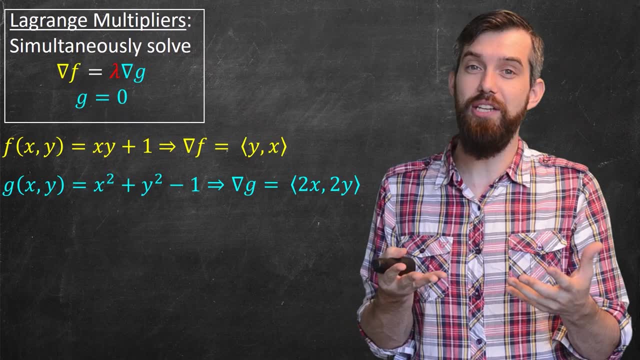 three equations in three unknowns. The unknowns are the x and the y and this new thing we've come up is lambda. So there's three unknowns, and x, y and lambda. But there's really three equations, because the first equation is a vector equation. Gradient of f is lambda, Gradient of g is: 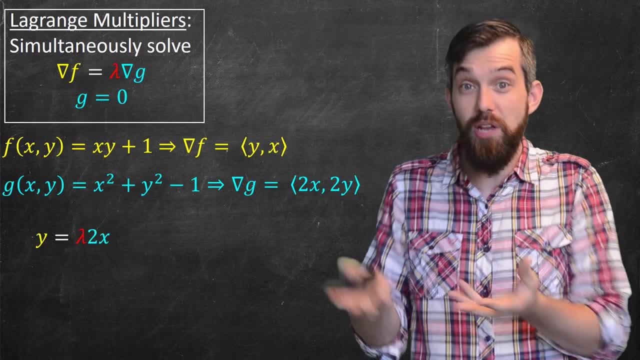 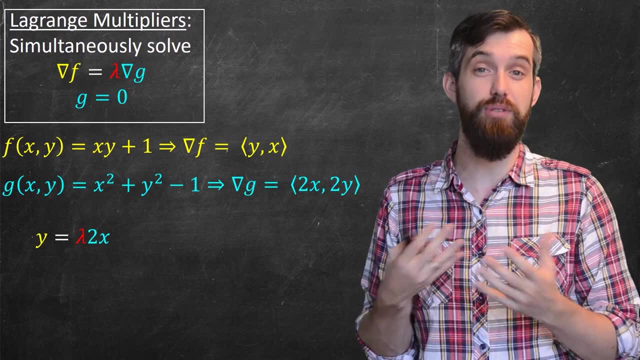 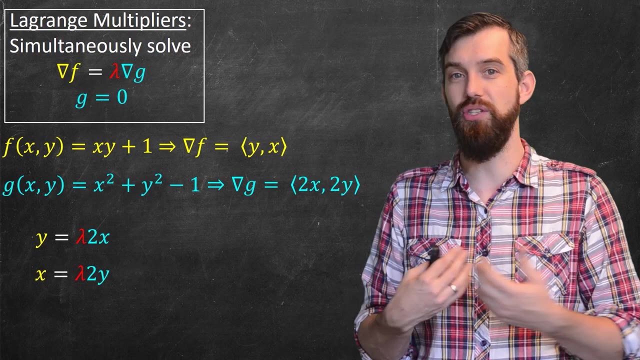 equating 2 to 2.. So the first components of that is the first component of gradient f is lambda times the first component of gradient g. In other words, just y equals lambda times 2x. Comparing the second coordinates of this, now I'm saying x is lambda times 2y. So the second component of 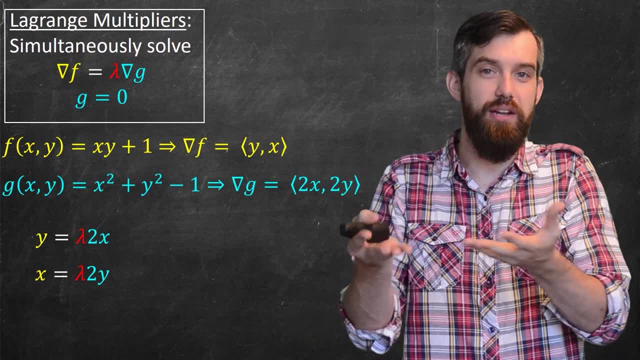 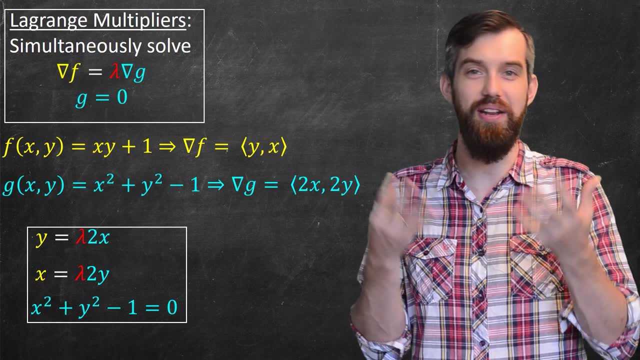 gradient f is equal to lambda times the second component of gradient g. And then my third equation is the good old constraint that we've always had: the x squared plus y squared minus 1 is equal to 0.. So these are my three equations. 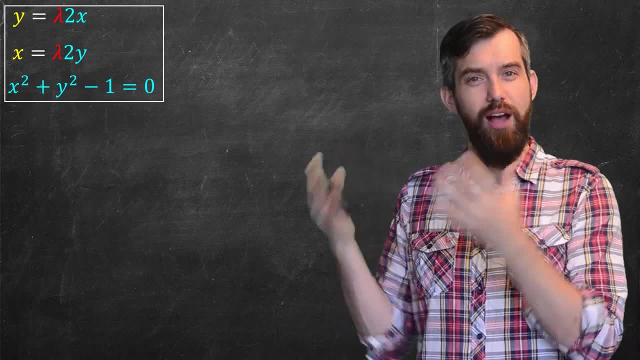 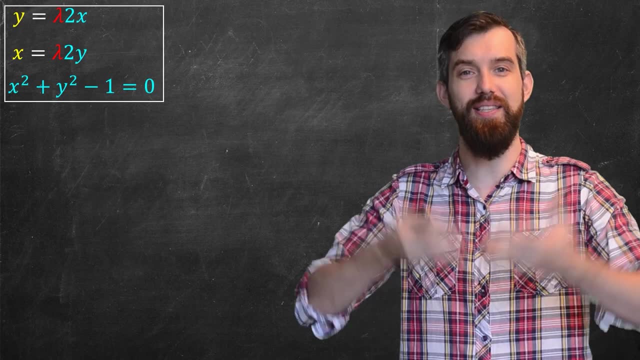 equations. Now, depending on your problem, the specifics of the algebra of solving these equations simultaneously, that might change. In this particular case, it's relatively straightforward. What I'm going to do is I'm going to take the second equation, x, equal to lambda 2y, I'm going to plug it into the first and that's going to give. 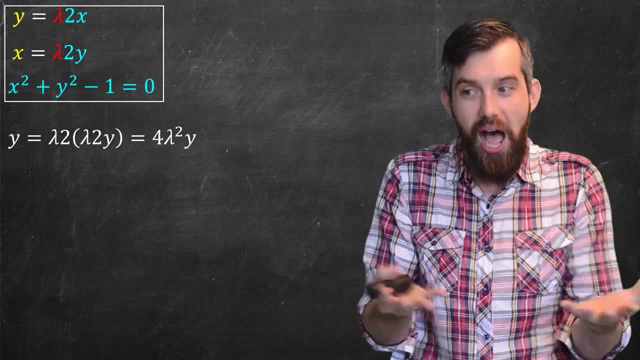 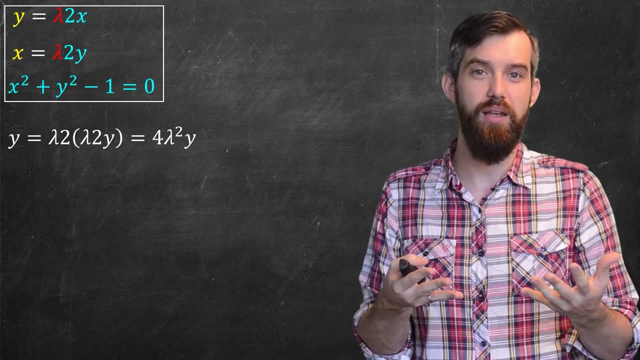 me the equation that y is lambda times 2 times the lambda times 2y. You put all that together, you get y is 4y squared times y. Now this equation has two possible answers. One solution is just that y is equal to zero. you just have. 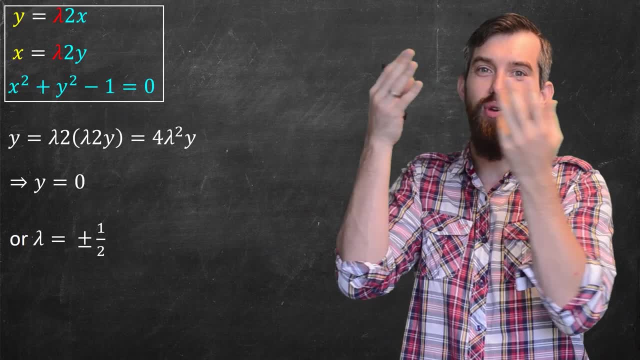 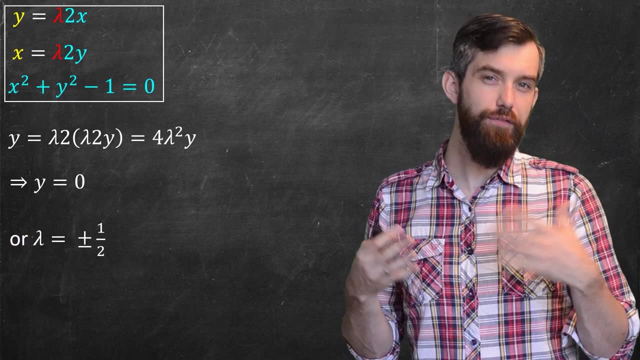 zero on both sides. If y is non-zero, then you can divide out by the zero and then if you solve that, you get. lambda is equal to plus or minus 1 half. Now, in the first case, if y is equal to zero, then reading off into the first or second, 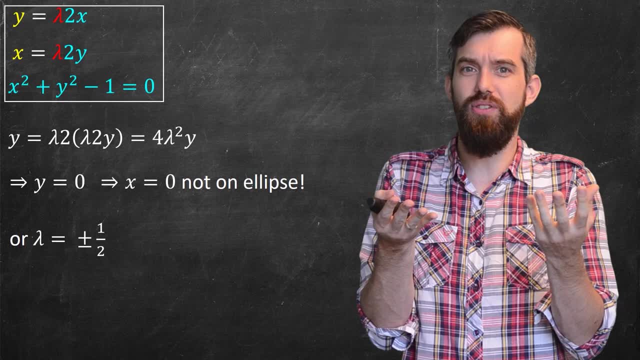 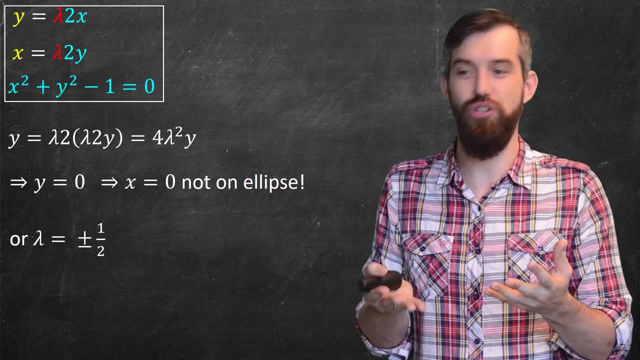 line you get that x is equal to zero and zero. zero was not on the original ellipse. the ellipse, x squared plus y squared, equal to one. so this is just not actually true. This is actually a solution that does not satisfy the third equation. So if I take the lambda, 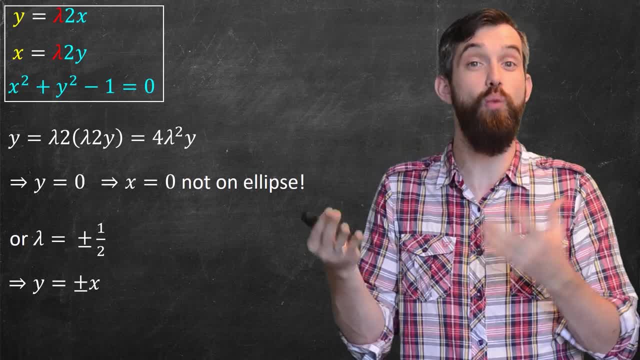 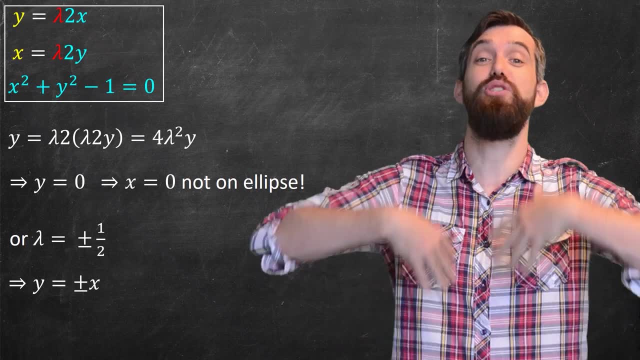 equal to plus or minus 1 half and plug this in, this tells you I have a relationship between y and x. y is plus or minus x. And now that I know this, if I take the y is plus or minus x and substitute it finally into that third, 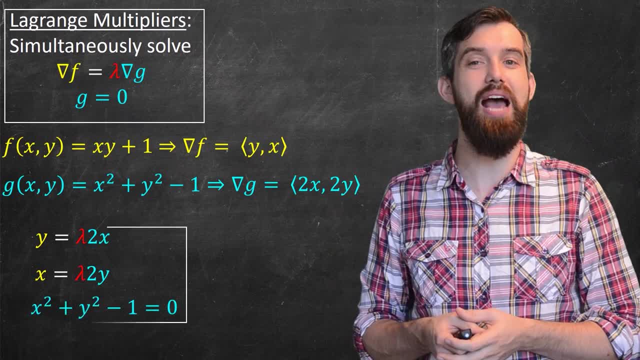 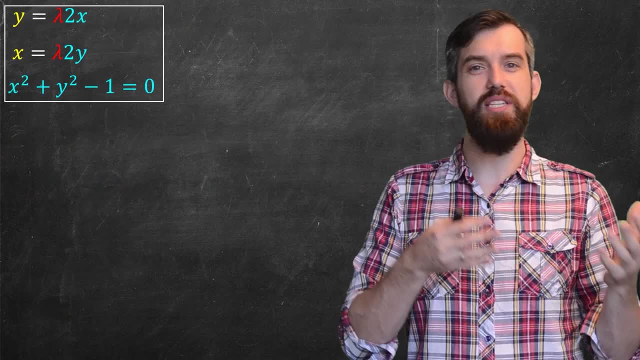 And then my third equation is the good old constraint that we've always had: the x squared plus y squared minus 1 is equal to 0.. So these are my three equations. Now, depending on your problem, the specifics of the algebra of solving these equations simultaneously, that might change. 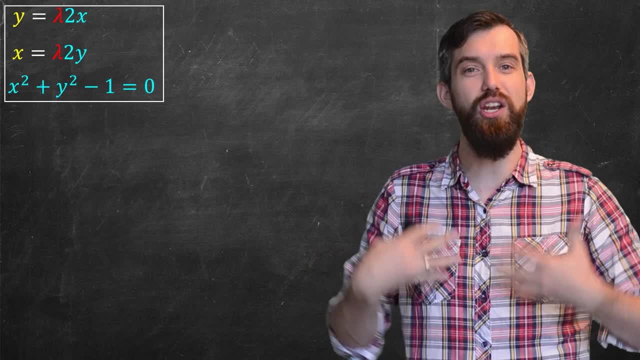 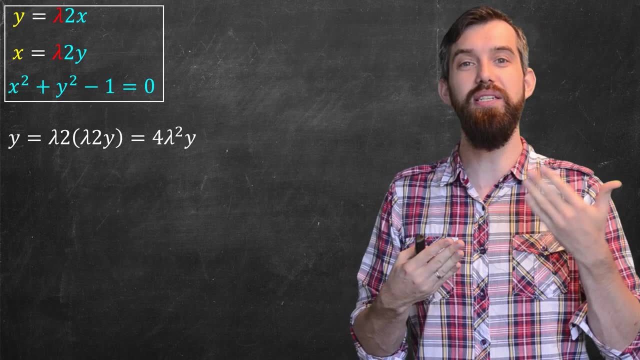 In this particular case, it's relatively straightforward. What I'm going to do is I'm going to take the second equation, x, equal to lambda 2y, I'm going to plug it into the first and that's going to give me the equation that y is lambda times 2 times the lambda times 2y. 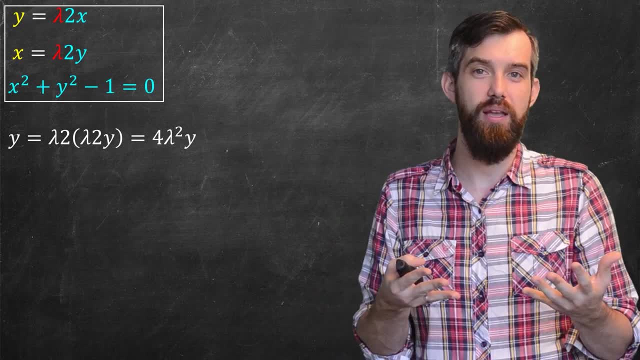 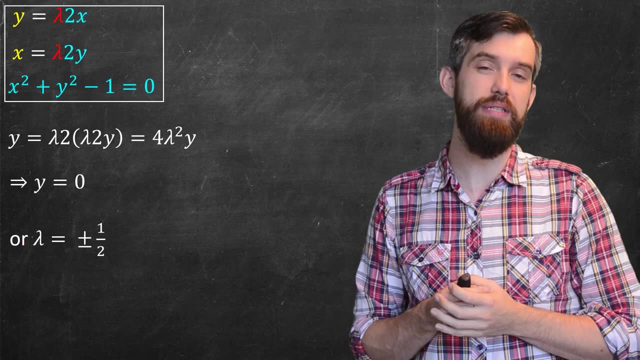 You put all that together, you get y is 4y squared times y. Now this equation has two possible answers. One solution is just that y is equal to 0. If y is nonzero, then you can divide out by the zero. 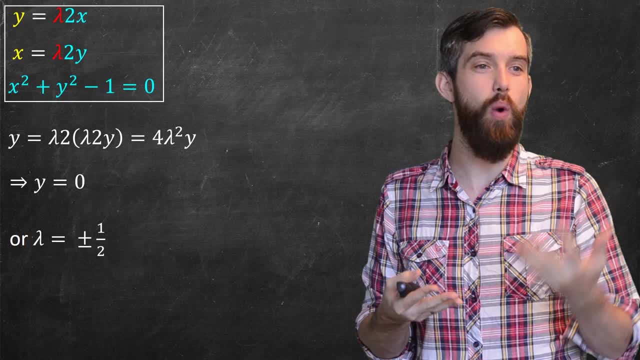 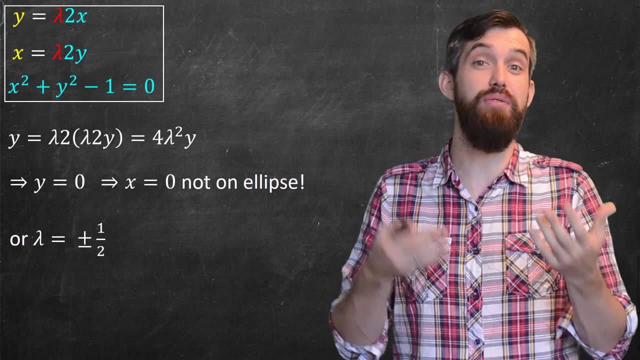 And then if you solve that, you get lambda is equal to plus or minus 1 half. Now, in the first case, if y is equal to 0, then reading off into the first or second line, you get that x is equal to 0. 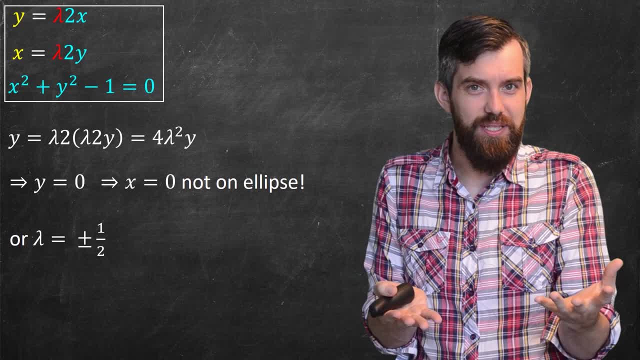 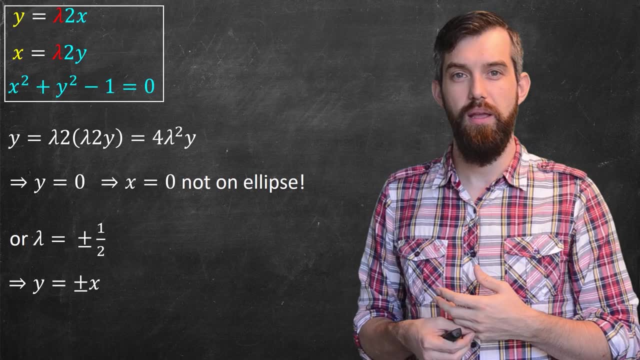 And 0, 0 was not on the original ellipse. the ellipse x squared plus y squared, equal to 1, so. So this is just not actually a solution. It does not satisfy the third equation. So if I take the lambda equal to plus or minus 1 half and plug this in, 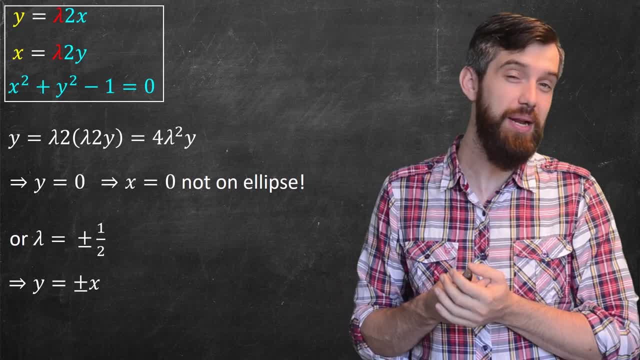 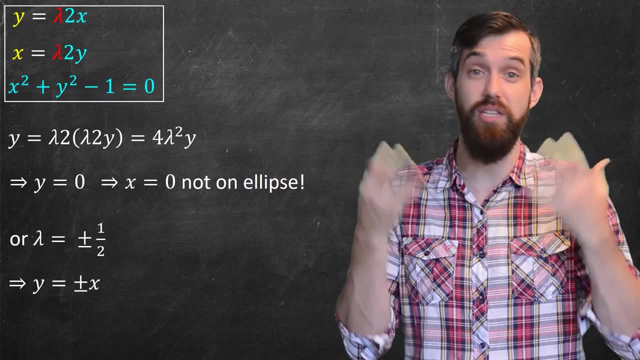 this tells you: I have a relationship between y and x. y is plus or minus x. And now that I know this, if I take the y is plus or minus x and substitute it finally into that third equation, into that constraint, I get x squared. 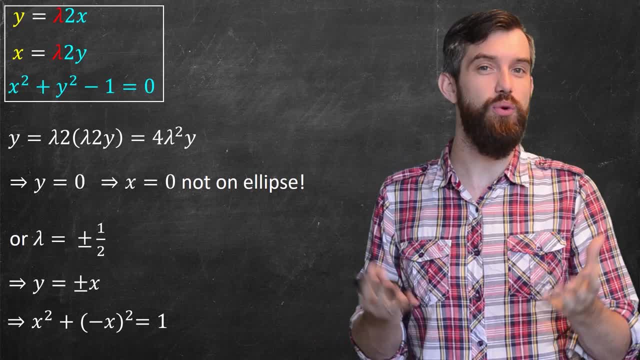 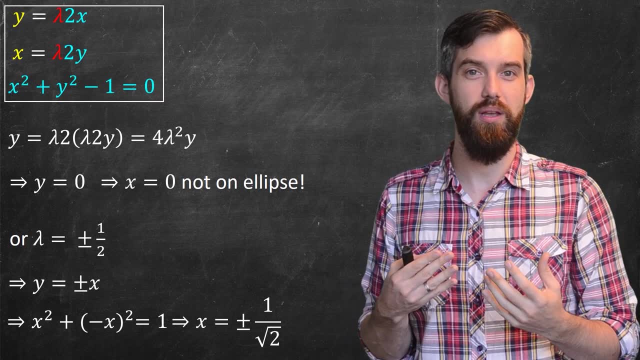 Then I get: well, minus x, all squared is equal to 1.. This tells me, 2x squared is equal to 1.. So x is plus or minus 1 over root 2.. There's really four possibilities here: x is plus or minus 1 over root 2.. 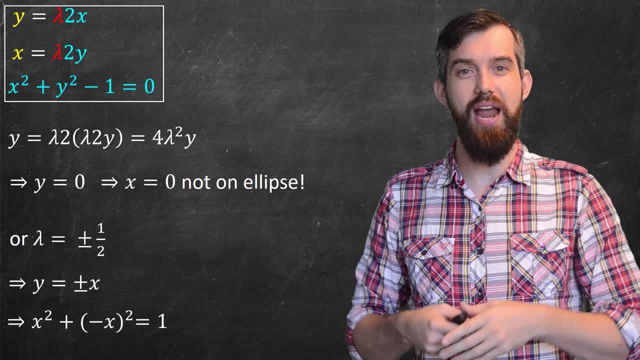 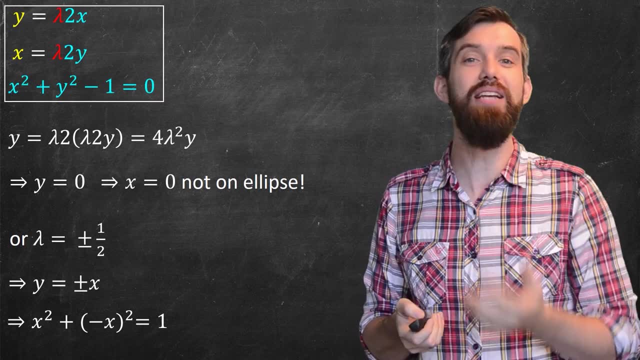 equation into that constraint. I get x squared, Then I get well, minus x. all squared is equal to 1.. This tells me 2x squared is equal to 1, so x is plus or minus 1 over root 2.. 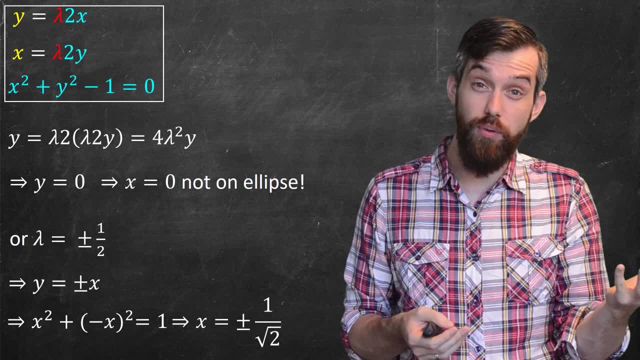 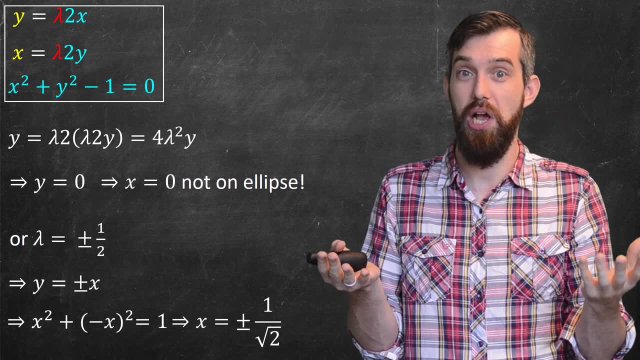 There's really four possibilities here. x is plus or minus 1 over root 2.. y is plus or minus those values, so also plus or minus 1 over the square root of root 2.. So there's four different possibilities for the x's and the y's. So I return back to. 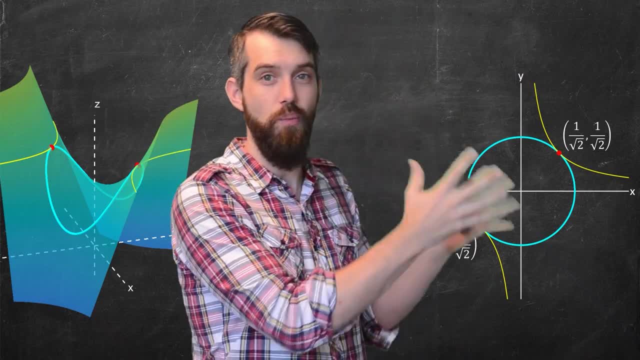 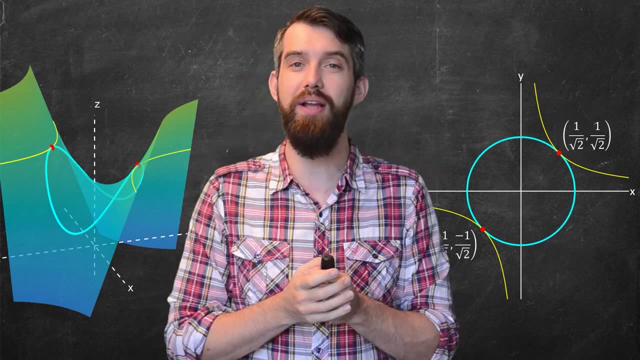 the geometry where I've got the graph of my function and where I've got my domain specified. And what I've done is I've taken two of those four points and what we can see is that for two of those four points, those do represent the maximums. 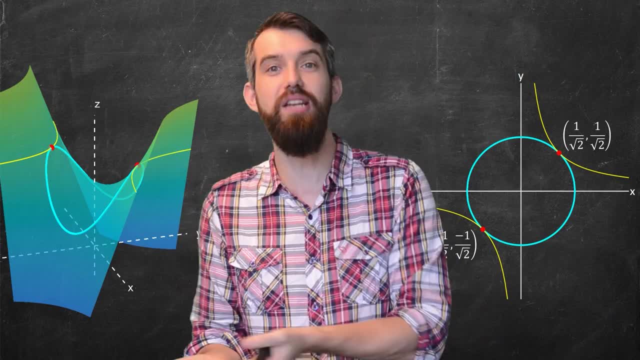 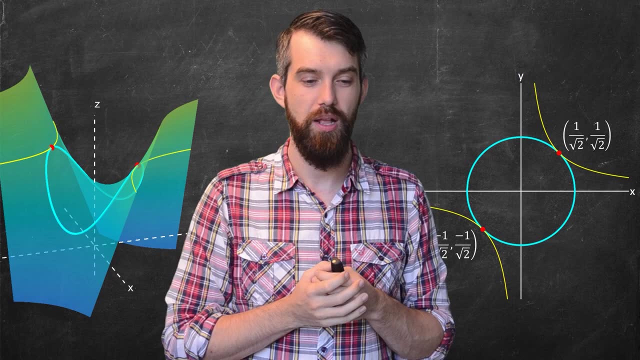 of this function. If you wish, you could plug these numbers into the function. you would get the value 1.5.. That is the maximum of this function, constrained to this particular equation. Likewise for the other two. well, they represent. if I shift the situation, I now 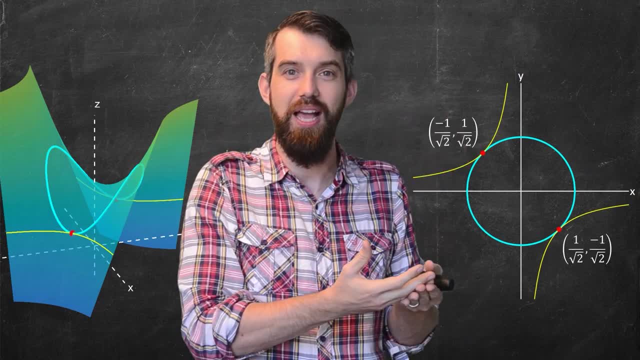 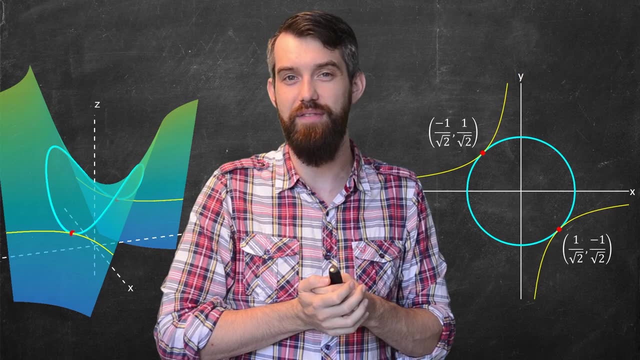 not ask for maximums, but I ask for minimums. They give you a slightly different pair of points and you get a different level curve. Now it happens to be equal to the height of 0.5.. And these two points are at the minimums, So notice. 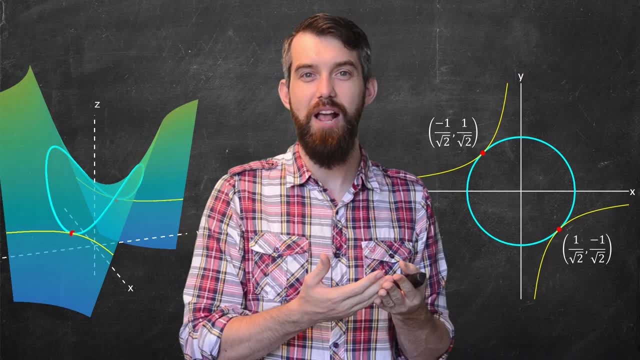 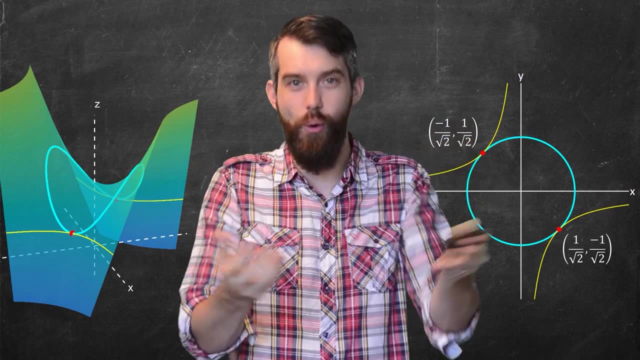 by getting those four points. I didn't know which was maximums and which was minimums. The idea of Lagrange multipliers is that this geometric analysis that we did gave a very nice extra equation. The gradient of F was lambda, gradient of G. That equation was in addition to the constraint that we 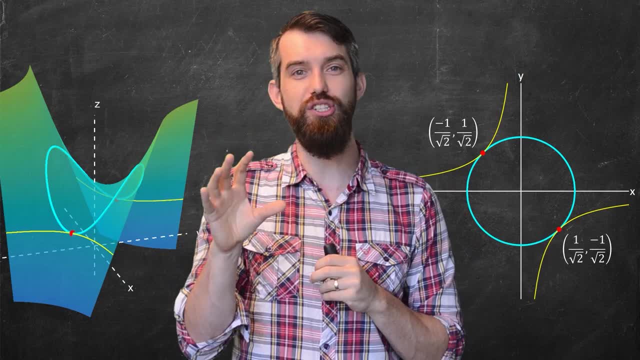 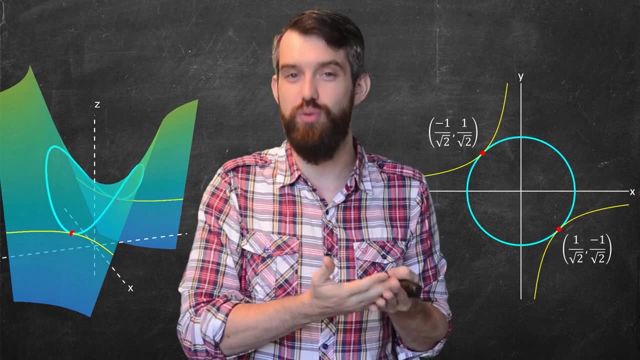 already had, that G was 0.. When I looked at those equations and solved them out, what they gave me were all of my candidates to be maximums or minimums. I didn't know which were maximums and minimums ahead of time. but if you then have a 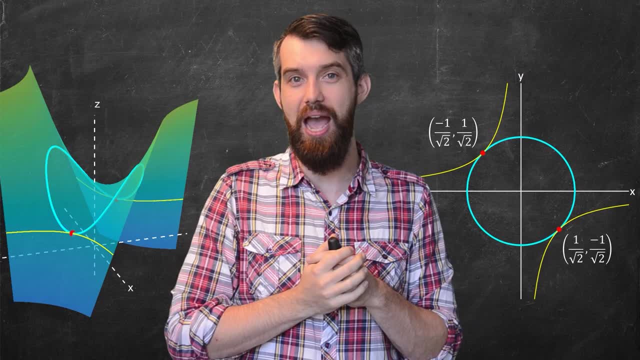 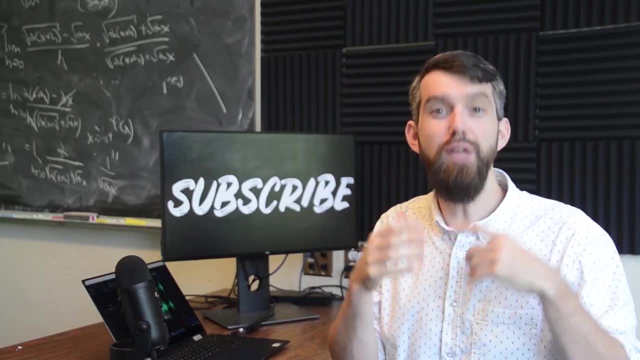 look at your function, at the points- in this case the four points that we had- you can see that two of them are going to be the same value in the maximum and two of them are going to be the same value in the minimum. If you have a question about 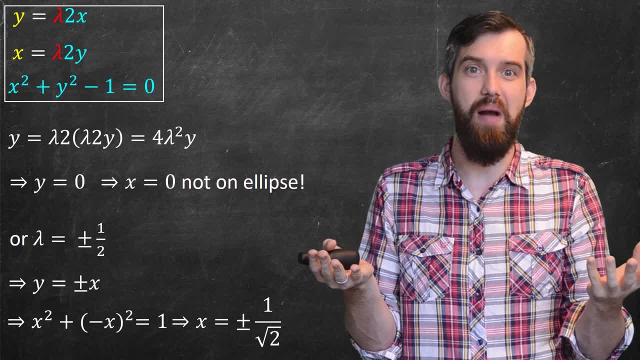 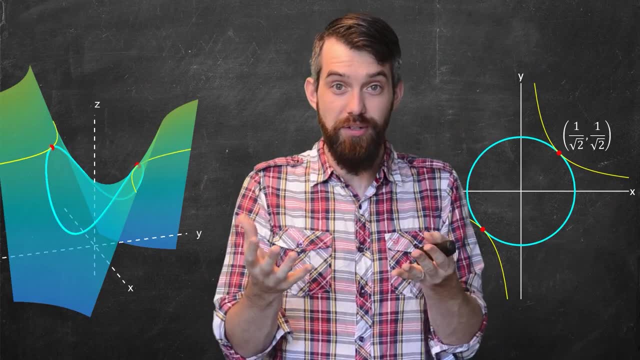 y is plus or minus those values, So also plus or minus 1 over the square root of root 2.. So there's four different possibilities for the x's and the y's. So I've returned back to the geometry where I've got the graph of my function. 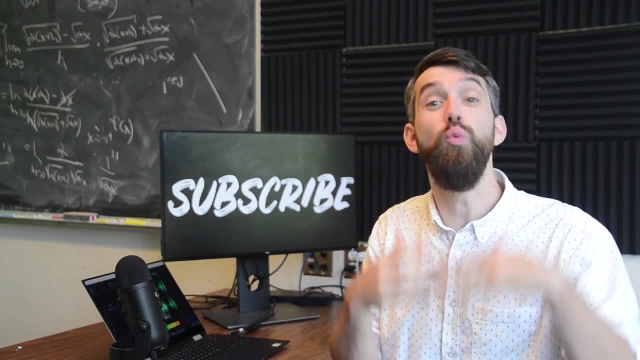 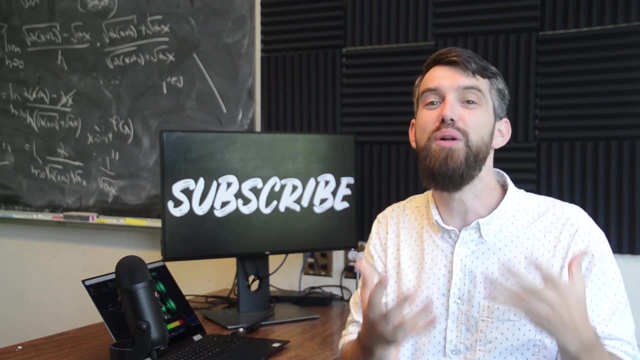 this video. leave it down in the comments below. We're all mathematicians here. We appreciate algorithms, so let's just help the YouTube algorithm out by giving this video a like. And finally, if you want to watch more multivariable calculus: 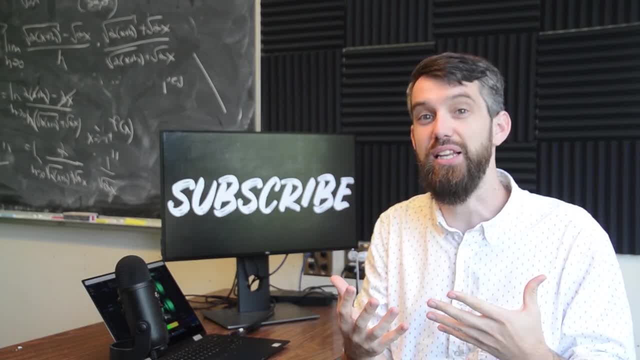 videos. this video is part of a larger playlist on multivariable calculus, so